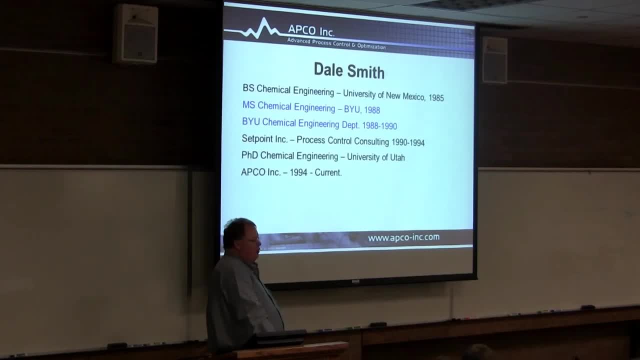 I was responsible for a lot of the automation in the lab over there. Before they used to have a baby network 90 system over there, We got that donated. Look at her shiver and shake. Now I guess they replaced it with something anyway. 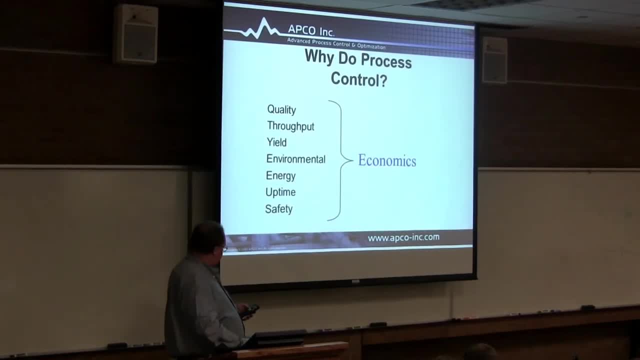 But anyway, that was pretty much it. That was kind of my contribution. I got some control classes while I was here. When I went to Setpoint I actually went all over the world and just about anywhere. I did a lot of Europe, a lot of time in Japan, Norway, Spain, Germany, Italy, France doing advanced control. 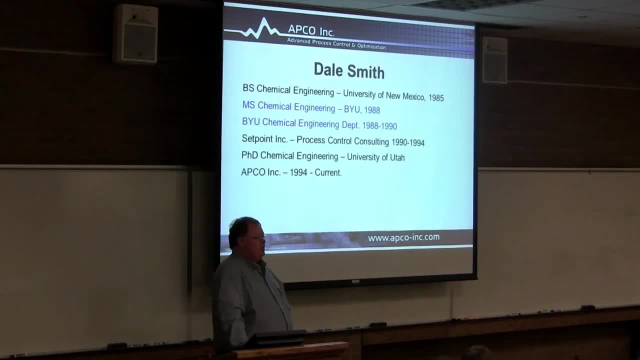 And what we did was fun stuff. It was good stuff. I remember when I was graduating in process- Even here in process control the chemical engineering was kind of an emphasis on process control- There really weren't a lot of companies that came to BYU looking for people in process control. 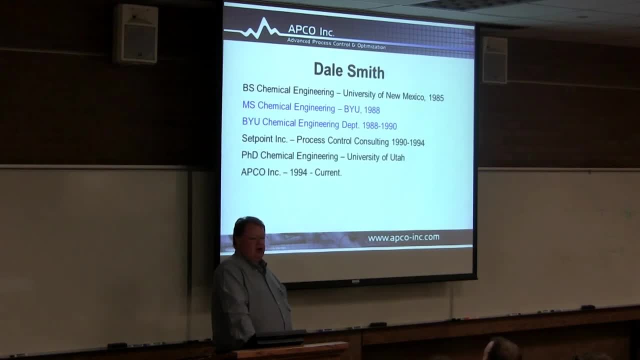 And they're probably still on it. BYU is not known as a great process control school. We think that's going to change. Dr Hedgren is fantastic. I'm thrilled to death that he's now a faculty member. down here There was a fellow that worked with me. 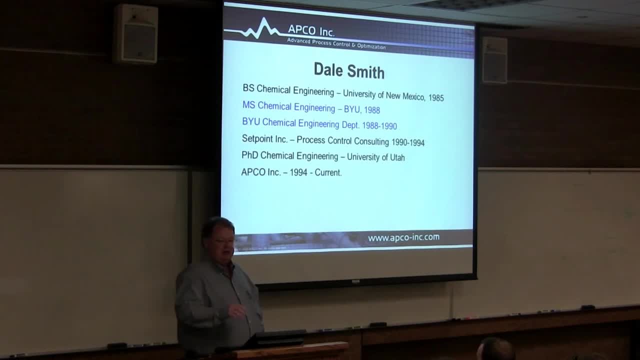 His name is Scott White. Scott's one of the smartest people I ever know. He's now my vice president of my company And he was just as close to a genius as I've ever met, And I remember when Scott and I left we had a passion for process control but not a lot of other people did. 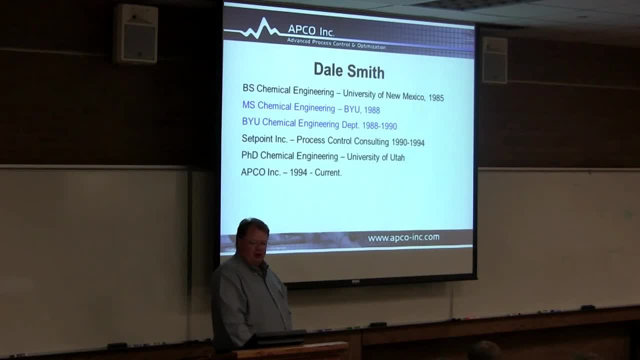 And so when we left, kind of the drive for the program died out And we've been begging the department for 15 years to try to get somebody in control, Dr Hedgren, is the result- not the result of us, but the result of the department doing that- 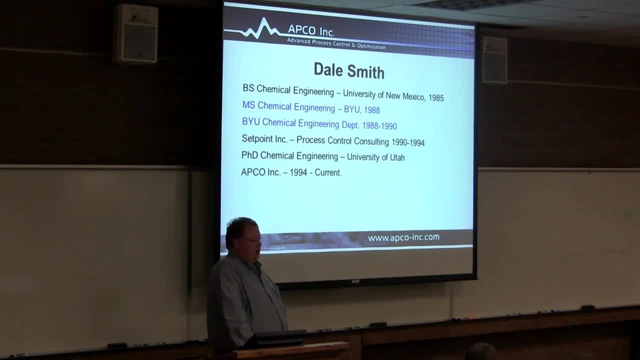 And we are just greatly excited and appreciative for that. Let me just tell you a little bit about process control. You guys said you're all seniors. Why do you think you're taking the process control class when you're seniors? Is it more applicable? 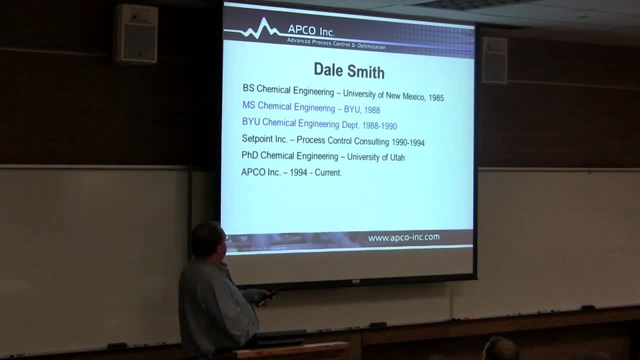 Is it more applicable? Let's go ahead and go through some of these slides and we'll take a look and see It worked out a little. Oh, There we go. The reason we do process control is it's almost always economics. 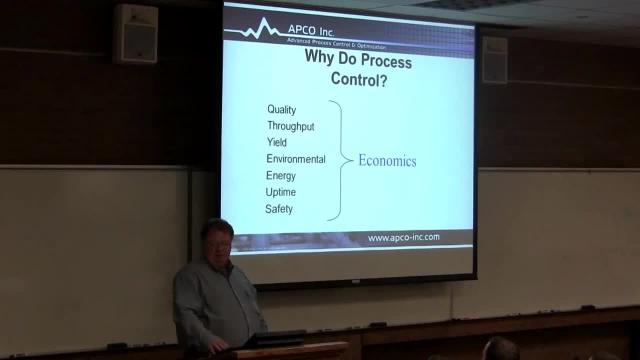 When you go out and talk about it. you guys have learned a lot about different kind of process operations, haven't you? You've got heat transfer, mass transfer. You're getting that right now. Separations, Thermodynamics, Fluid dynamics. 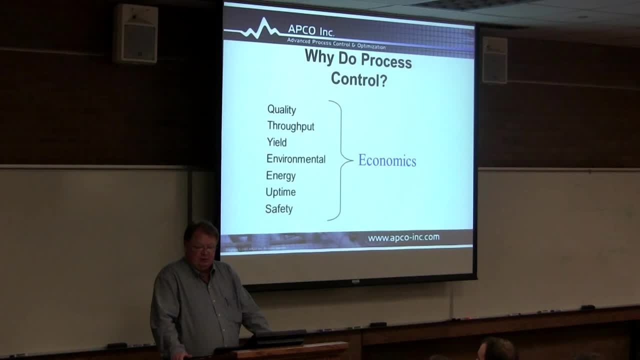 Kinetics Reactor design. Okay, What happens when you go out in the real world, You start using all that stuff. Where does it go? Put it in a plant somewhere, Don't you think? I mean, it's great to have it in the computer. 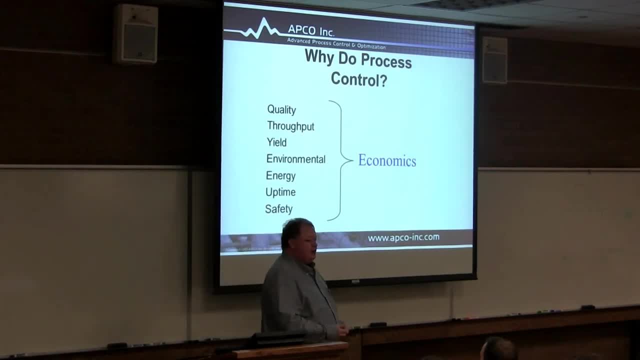 I know you guys are all computer gurus, But when you go out in the real world do you think you mess around in the computer all the time? Is money made in the computer part of it? The money is always made when the plant is built, right? 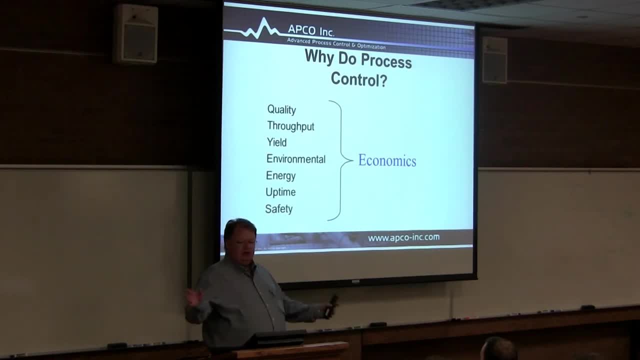 So the operation is not a computer. The operation are a bunch of pieces of equipment and stuff like that. So all of the work you've been doing up to this point has really been so that I can design something, So I can build something. 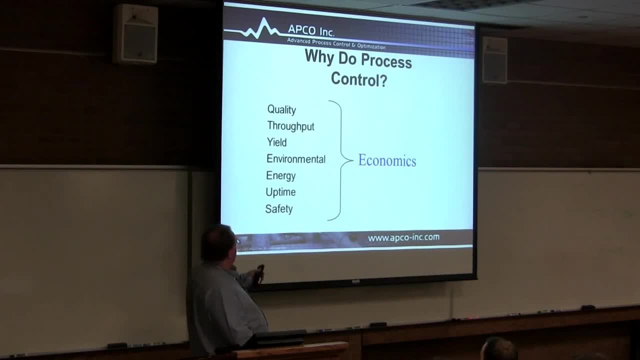 I can make it work right When you do that. you want it to have good quality. You want it to have great throughput yield, be environmentally conscious, energy conservative. You want to have great uptime. You guys know what uptime is. 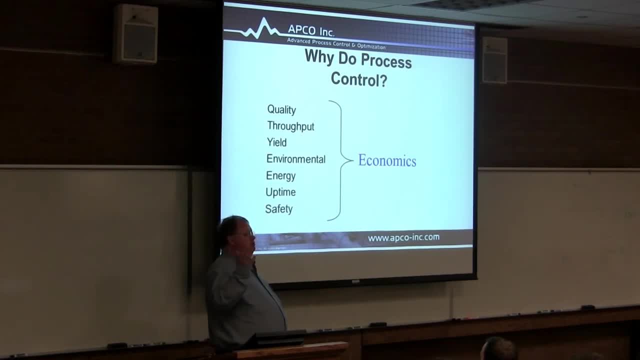 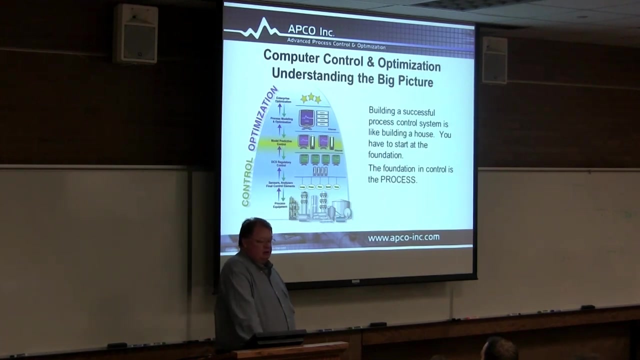 How much time it's actually running. Yeah, the fraction of the time it's up. So you want to keep it up All the time. All right, Much possible. And safety: You want to do it safely. Okay, Building a plant or doing process control or anything else is almost always the same. 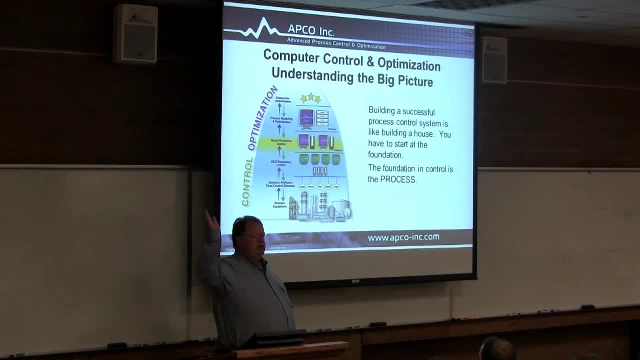 Who here has had any experience in construction? Any Who's seen a house built. What's the first thing they do when they build a house? They dig, What do they put in that hole? Basement, They put up walls, They put in a good foundation. 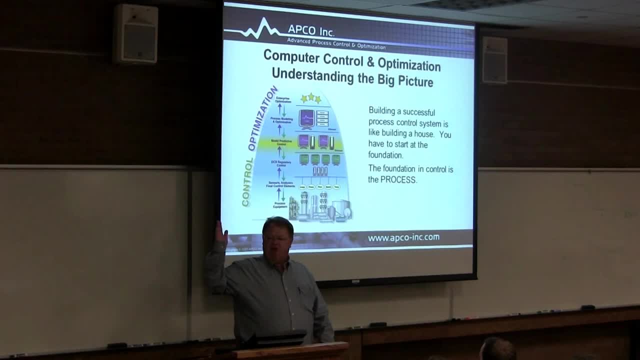 They put on a good floor And then they start working their way out right. So this is kind of like: Come on, that's a great place to be My back up there. So this is very much like what we do in chemical engineering. 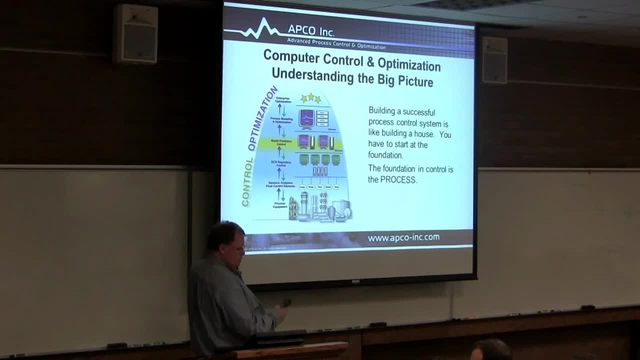 You guys have gone through all these classes: Reactors and distillation columns and tanks and towers and pumps and pipes and all the other stuff. By the way, when I was around here, I had a lot of fun. I had a lot of fun. 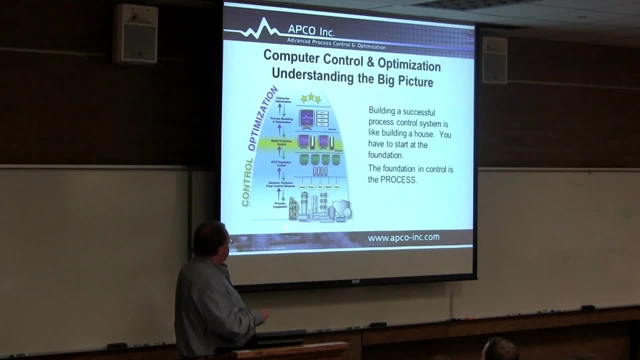 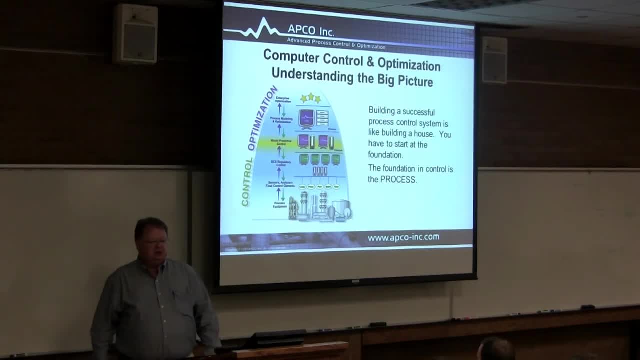 The reactors and distillation columns and tanks and towers and pumps and pipes and all the other stuff. By the way, when I would drive by refineries, you guys driven by refineries, Aren't they sexy Us chemical engineers? when we go by a refinery, we get excited. 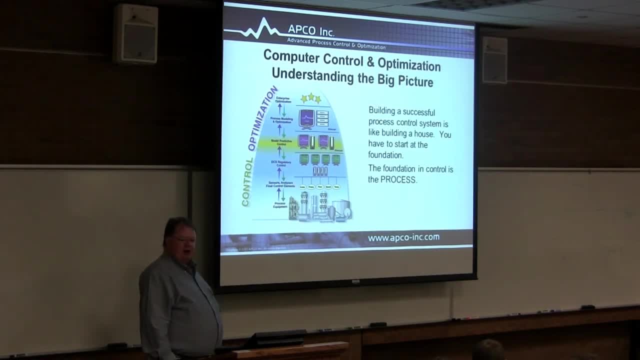 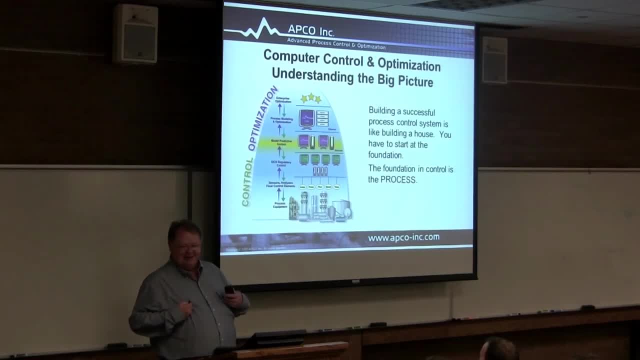 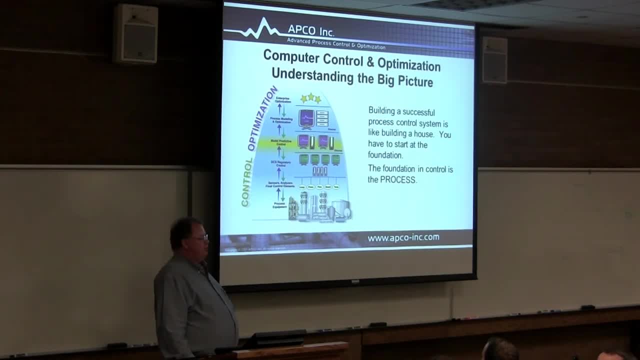 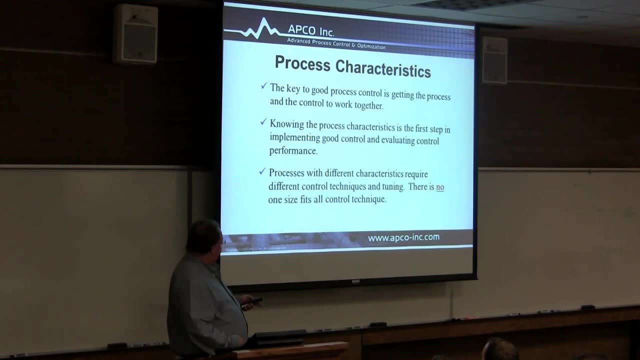 What do you put on? a foundation, A frame In this case? you're going to put on some instrumentation, because, as good an engineer as you are, you think if you just put in pipes and all this other stuff it's just going to run. Is that what happens? 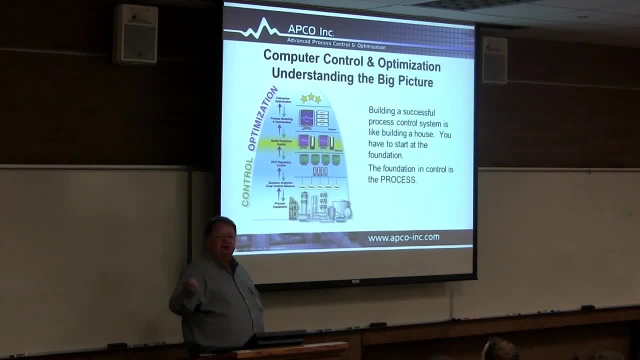 You just put it in and bat your eyes or blink or snap your fingers and all of a sudden there's stuff running through it. Is that the way it works? No, you have to have instrumentation If you're going to drive a car. do you want a speedometer? Do you want brakes? Do you want a windshield? 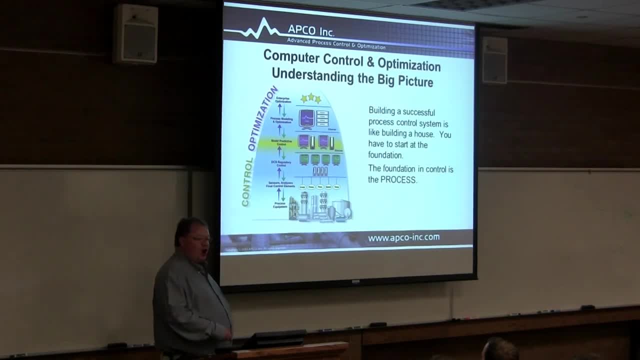 Do you want to see what's going on? It's all great that there's a car, but it's probably about wheels on it. you know You want tires, a windshield, stuff like that. We've got to be able to see what's going on. 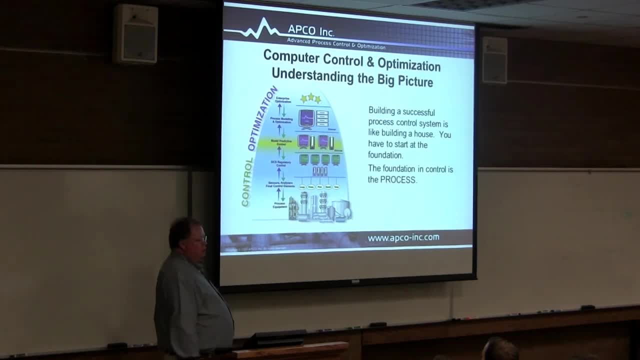 Above that, we do what we call regulatory control. Regulatory control controls the basin. Does your car have any regulatory control on it? What is the regulatory control? Any ideas? Go ahead. Temperature, Temperature, Yeah, So does your car overheat? 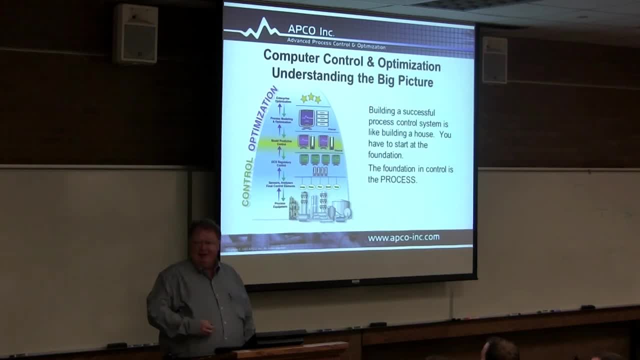 I heard she smokes a lot. Yeah, Smokes a lot. I have a daughter that Her car just She overheated last week so I had to go save her, You know anyway. so that was fun. I used to be a mechanic, so that's how I pay for my undergraduate education. 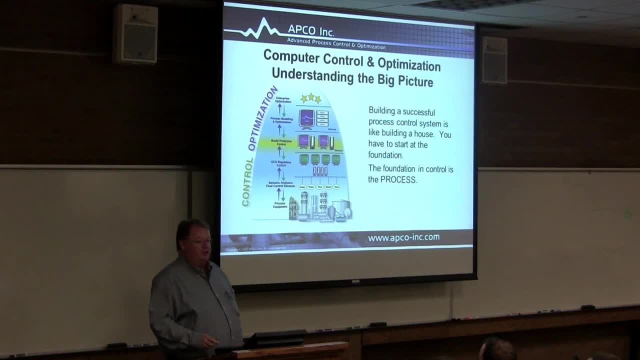 Anyway. so yeah, we don't want our car to overheat. That's bad, you know. For me things are either good or they're bad. Bad. good: The car, The regular heat, The total heat in the car. 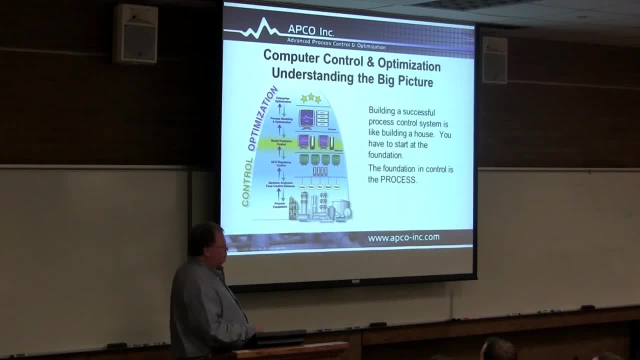 Good, Okay, All right, We have to have instrumentation. We have to be able to sense the temperature. We have to be able to know what's going on. We all want to know how fast we're going. We all want to make sure our battery's not going dead. 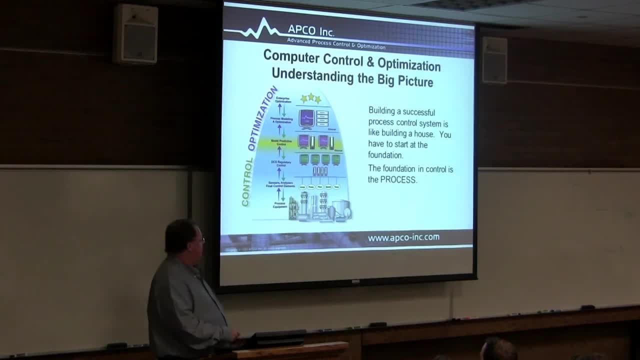 We all want to do all these different things in the car. We do the same thing in the refineries: Make sure that the level of the tank's not too high or too low. We don't want it overflowing. We don't want to run it empty. 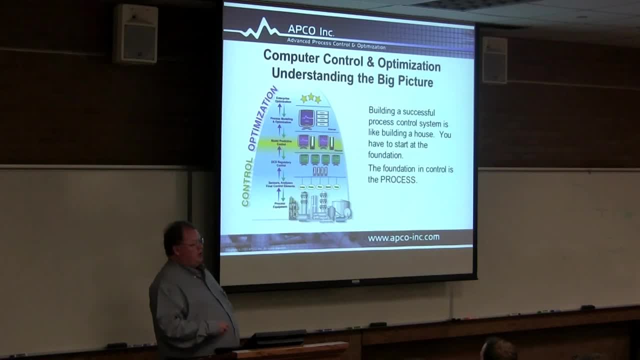 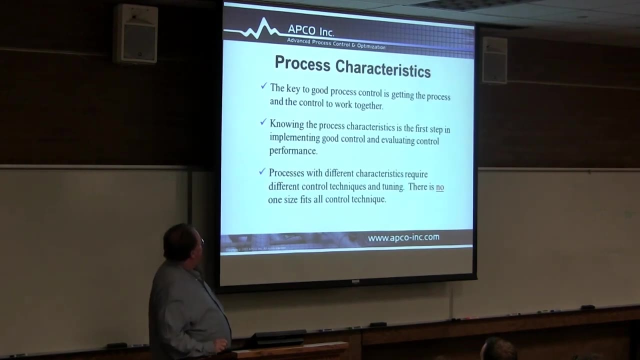 Right, Pretty straight and simple stuff. Okay, What Dr Hedgren wanted me to concentrate on today is how you use your engineering skills to be a good process control engineer. Let me just tell you right now that the key to good process control is getting the control. 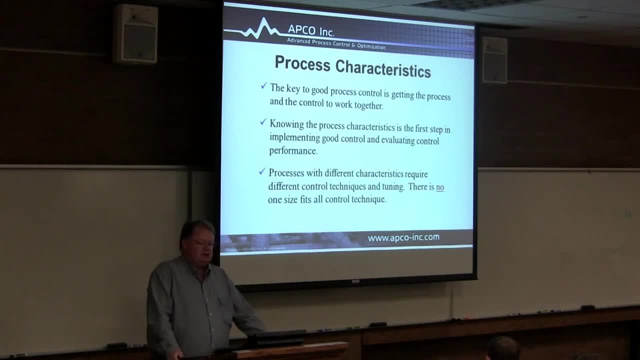 and the process to work together. The key word in process control is process. If you understand how the process works, actually, the control becomes very easy. Okay, You guys may think that's kind of odd right now, as you're starting to study Laplace transforms. 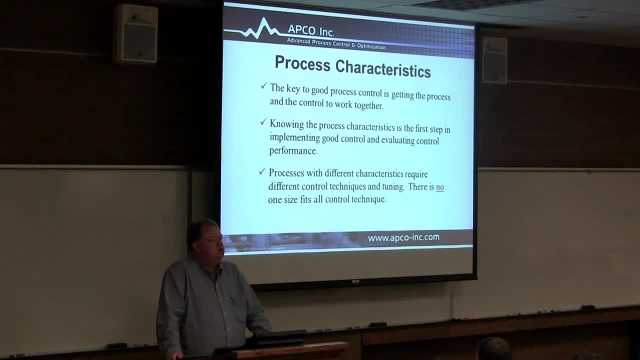 Why do you study Laplace transforms? Anyone know Who's in government? No, Bill's character, Bill's character. You know, I have a dog's dog, I have a dog, I have a dog, I have a dog. 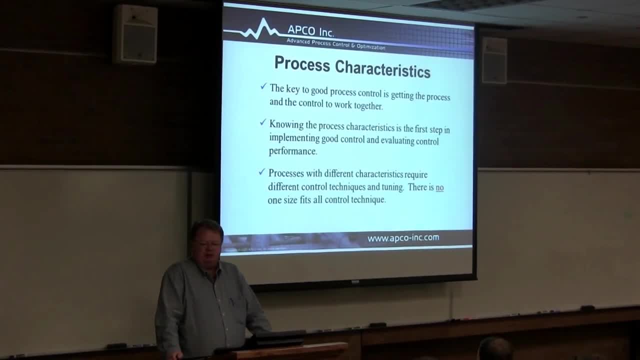 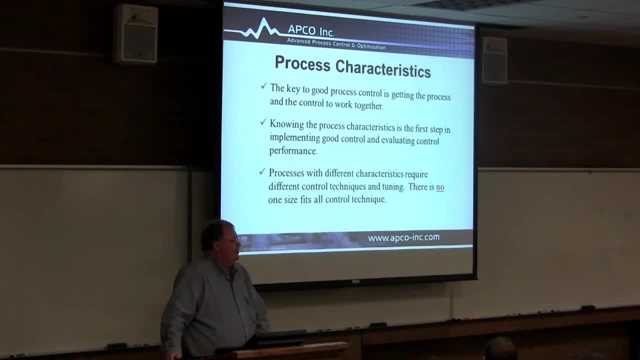 You want my dog, You want my dog, Right? You know, it's got got gets what's good and it's got got some good genies out there. You like cars, You like cars, You like right, We like big cars. 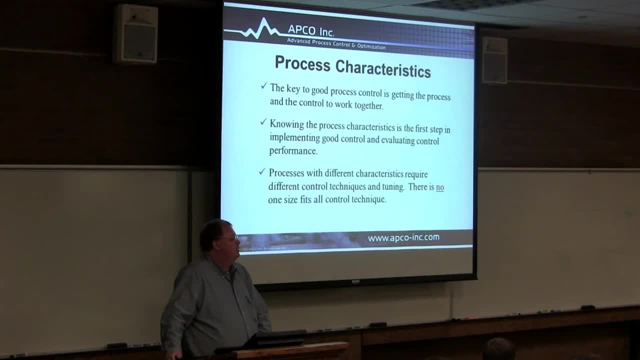 We like big cars. We like cars. We like about half the size of the car's narcotics. We like about one Andrea, We like about one flips. We like about one. This is about like 25, say, adults, old corp och 20 grand. 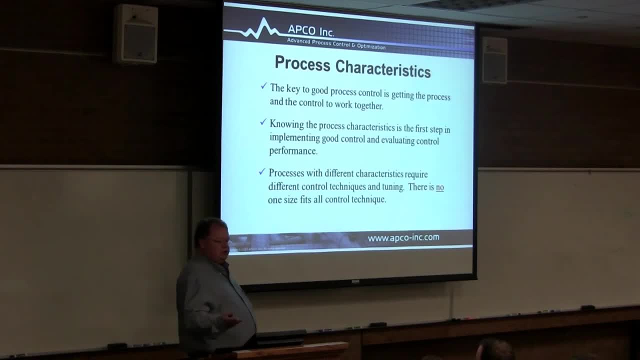 Do you like the plug for that van Wow? Awesome differential equations. who likes solving ODE's? Ooh, ooh, okay, turns ODE's into algebraic equations. Which would you rather solve, an ODE or an algebraic equation? 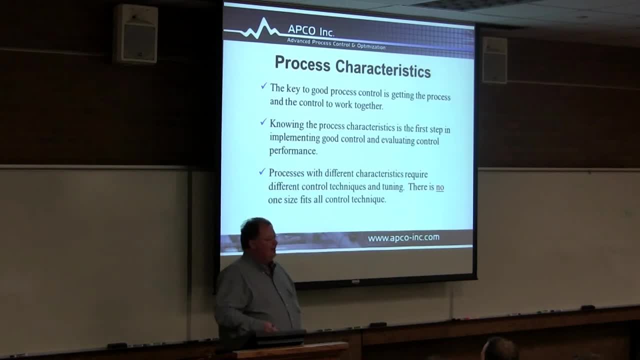 Yeah, yeah, yeah, that's what I'm talking about. So just know why you're doing it okay In the real world when you go out and do process control, like I have for the last 25 years. I haven't done no false transform in. 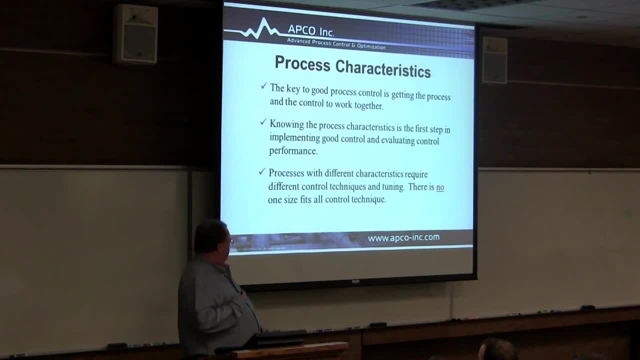 I've probably done five in the last 25 years. okay, So, but for the stuff that you're doing right now about learning about modeling of processes and stuff and characterizing processes, you kind of need to know what's transform, okay. 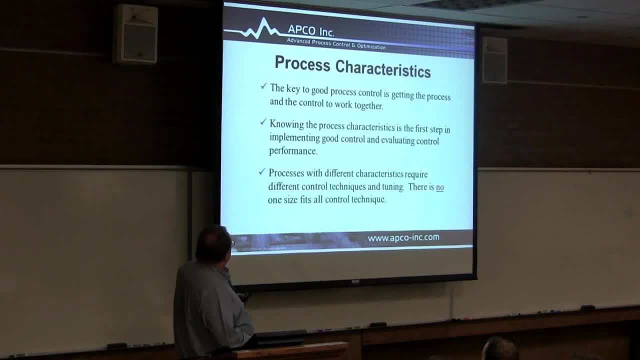 So it's a useful tool. Knowing the process characteristics is the first step in implementing good control. Processes with different characteristics require different control techniques and tuning. There is no one size fits all tuning technique. okay, So what's the key to getting good process control? 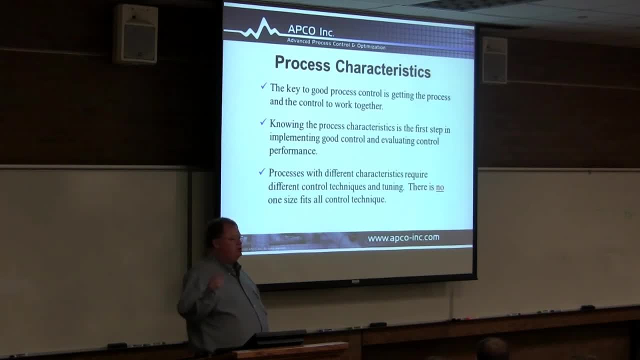 Understand the process. So here at APCO I've got a company, I've got positions open. okay, I have a hard time filling those positions. Why, First of all, I prefer to hire chemical engineers? Why do I prefer to hire chemical engineers? 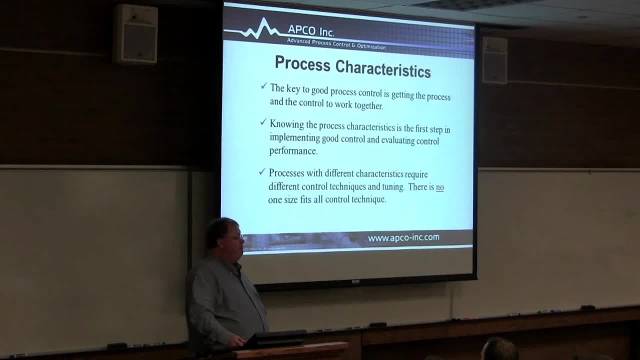 Because you're one of them. They have exposure to more processes than any other engineering field. okay, My second on the list would be mechanical engineers. So if I want to control a distillation column, who would I need to go to? A chemical engineer, right? 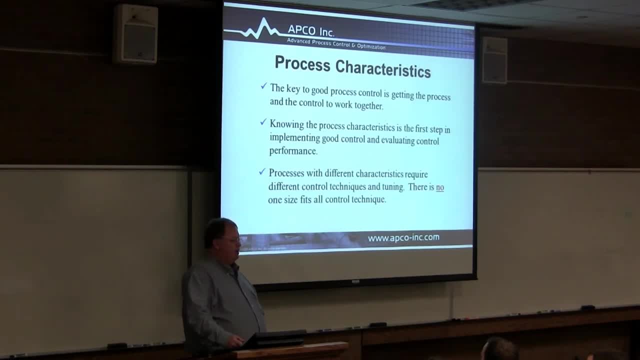 Or a reacting system. who's going to be best at that? Probably a chemical engineer. If it's a fluid flow or a pump or a heat exchanger or a mechanical system or a manufacturing system, would a mechanical engineer be good? 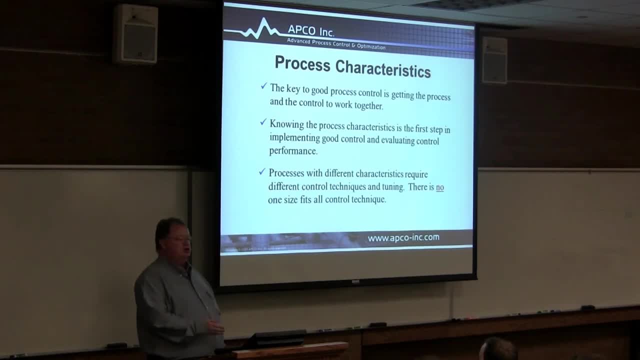 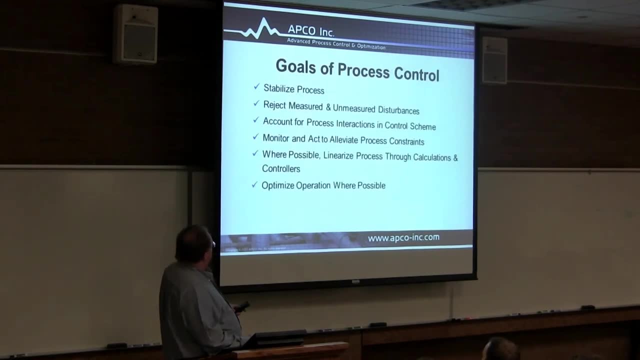 Absolutely, absolutely okay. But can a chemical engineer do those kind of systems? Yes, okay, so there's more breadth. I should be proud of that. that's one of the things. yeah, The goal of the process control is to stabilize the process. 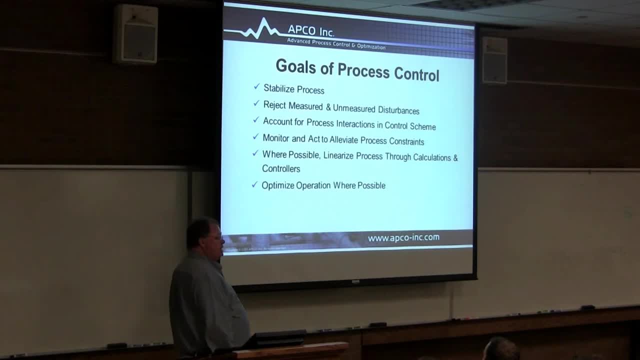 reject measured and unmeasured disturbances, Whatever you do in your design, in heat transfer or chemical kinetics or whatever, except for maybe I think they have a few minor problems, but almost everything you do is what we call steady state right. 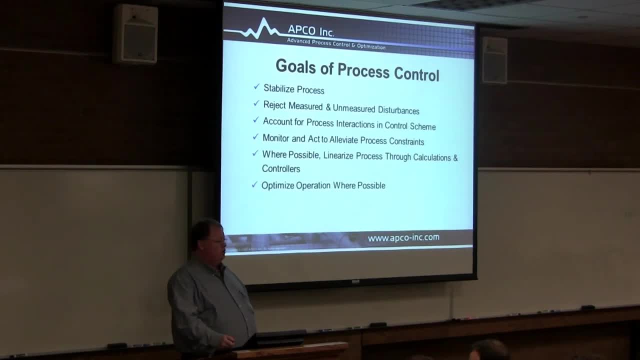 Design a CSDR, steady state, PFR or PFR, PFR. Hey, hey, hey, you guys are my uberos. All right, that's it. I'll pass the entrance exam to APCOE. you credit me for that. 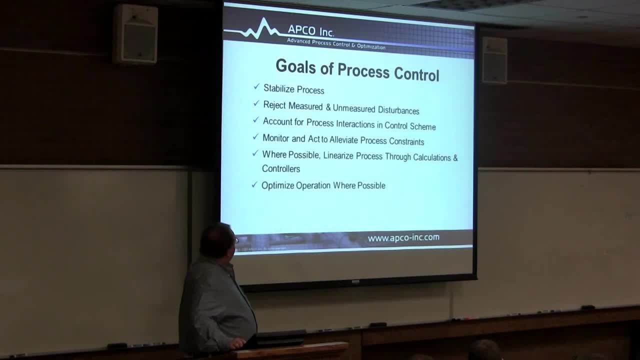 All right, that's not real hard, okay. All right, all right. So anyway, a plug flow reactor, any kind of thing like that. it's all designed around steady state. How many processes do you think actually run at steady state? 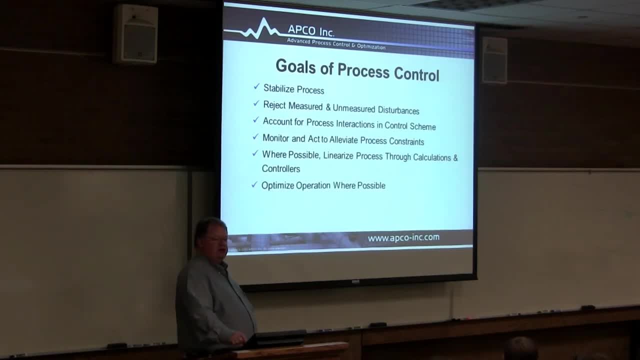 Zero, Zero, none, okay. So they design them around steady state. This happens all the time. They made me big bucks to go out with refineries, the chemical companies, things like that, to do P&ID reviews. You know what a P&ID is. 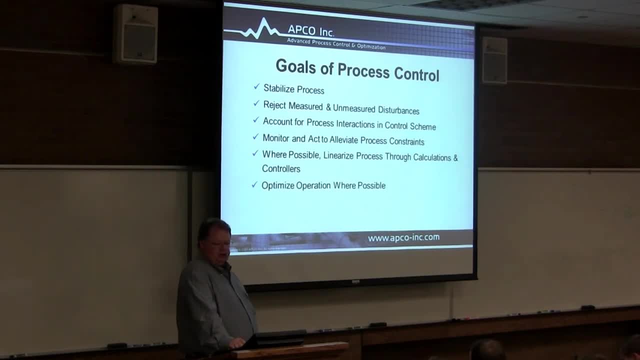 Process and instrumentation diagram. They say: tell us what's wrong with the controls. And the guys that design the controls are the guys that do all the steady state stuff. And they say: you know what? I can control the vapor pressure on this front. distillation column. 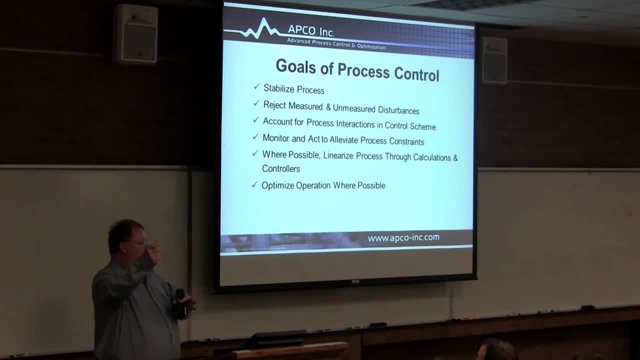 because it's connected all the way down through the process to this end tank. So I'll control the vapor, the pressure down there, and that controls the whole thing. And I go, okay, and I shake my head, I say shame, shame, shame. 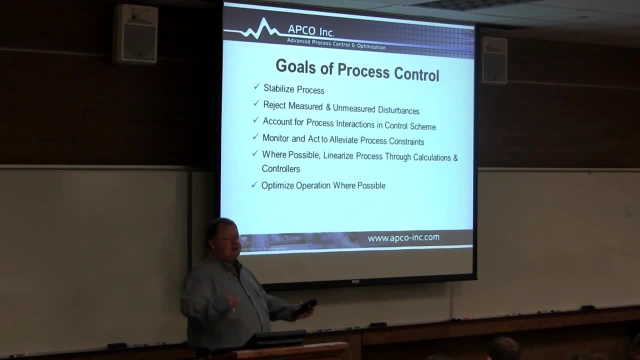 No, I don't really say that, but I think it, You know. And then they start criticizing me. Now you see how the whole thing goes, So you have to understand about dynamics. It's difficult for me to say hey. 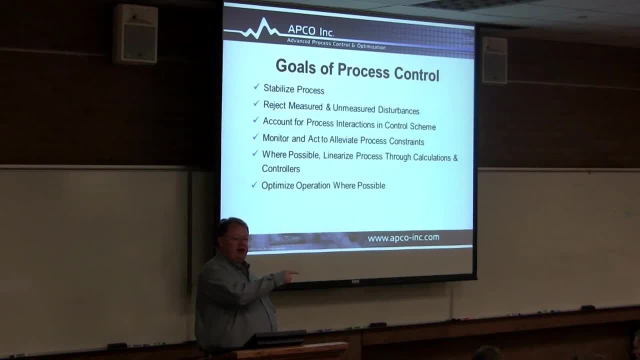 I'm gonna control something where, if I see a variable now, I'm gonna make the change a half an hour from now, when I see it at the end of the pipe, and it's gonna be able to get good control of the front. Does that make any sense? 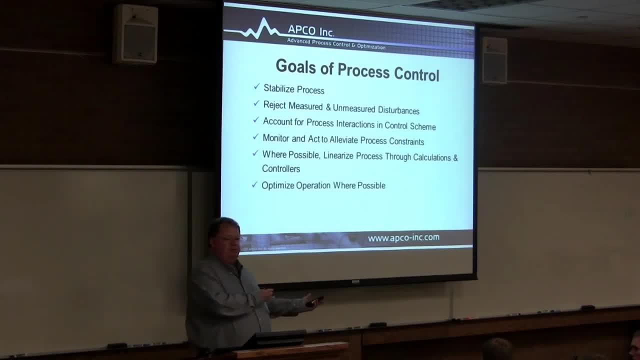 How many of you ever had a car that had a carburetor on it? It's gone from like 98% of the class to one guy. That's how old I'm getting. I'm telling you it's bad, it's really bad okay. 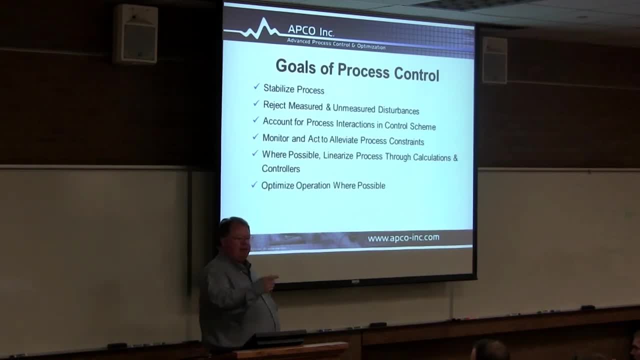 The carburetor gets a little, you hit the gas hard right at the front end and what happens? Nothing, Nothing. If you hit the gas hard on the front end of the refinery, nothing happens. what are you gonna do? You're gonna hit it harder, right? 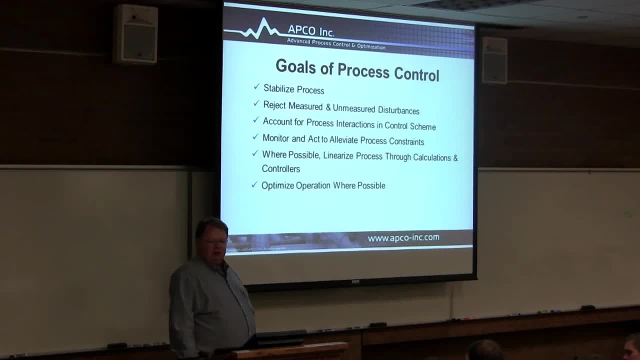 You're driving your car, you push the gas, nothing happens. what do you do? Push it harder, Push it harder. So then, when it finally catches, how fast are you going Too fast? A little too fast, okay. So understanding that and just understanding the relationship. 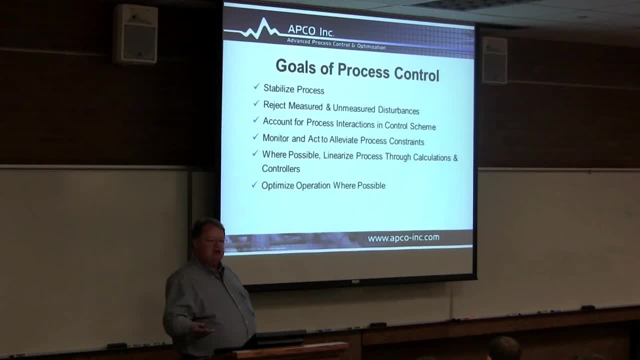 between when I make a manipulated variable change, when I make a change in the process, and how it affects the process, not only at steady state, but between now, and steady state is an important concept, right? okay, That's what you guys are learning about, okay. 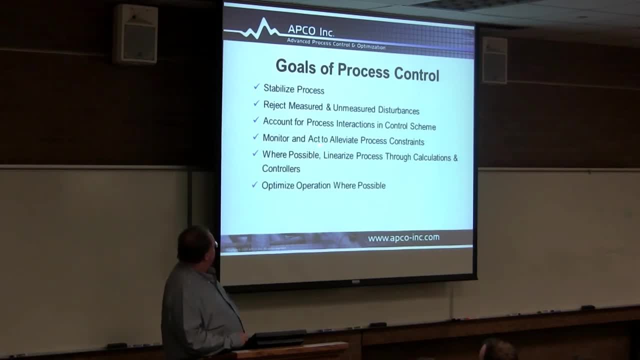 It's a very important thing. okay, We account for process interactions in the control scheme. How many of you guys have ever been in a home with two showers, Or in the shower and the toilet? You're in the shower and the toilet flushes. 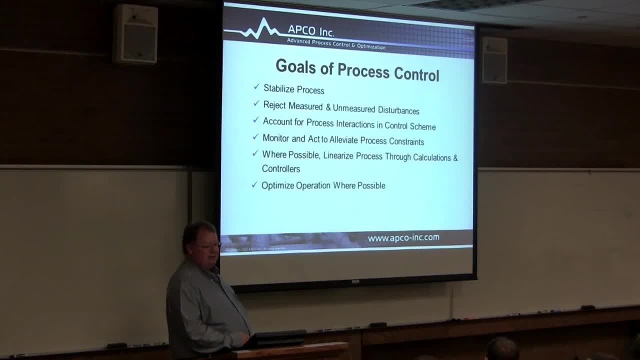 what happens to the water temperature? Ice cold, Huh, Ice cold. Who said ice cold? Who said ice cold? Not unless your toilet's hooked up to the hot water. No, Wow, I wouldn't want that. All right, that's not good. 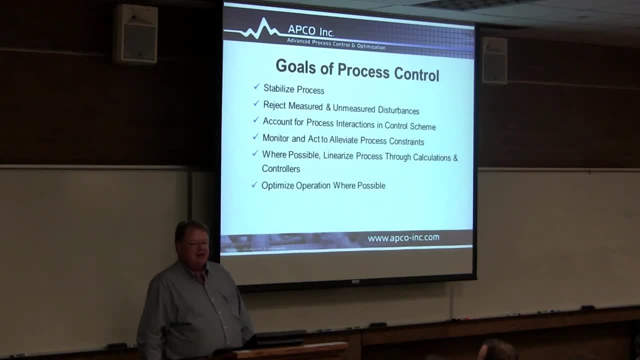 So being able to reject that interaction would be nice. So being able to reject that interaction would be nice. So being able to reject that interaction would be nice, Wouldn't it? okay, That's what we do. So we say, hey, look, we know if this is gonna change. 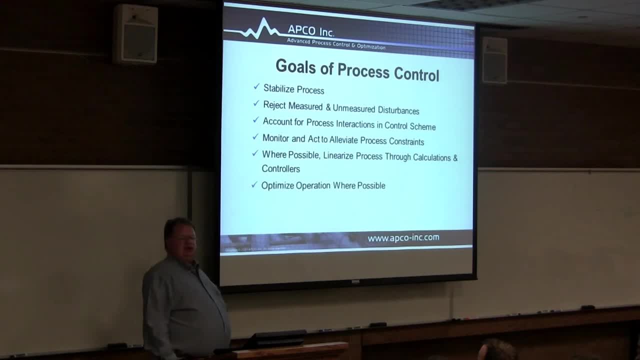 this is gonna change and we can take that into account. How do we know what's gonna change? Intuition, intuition, oh intuition. That's a good guess. Are you sure you're a senior? Go ahead, That's experience in the plants. 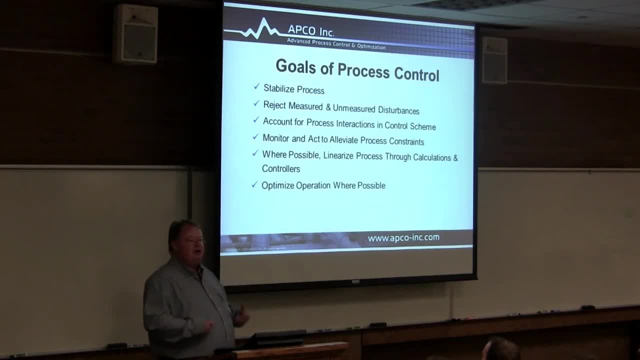 That's experience in the oh. we're better than that. We know what's going on with the process, right? So if I flush the toilet, why does the water get hot in the shower? The water pressure drops on the cold side, right. 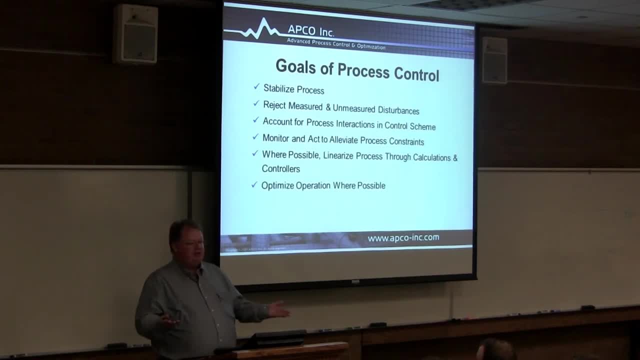 So there's more hot water than cold water, because the pressure is the driving force for flow. So the water gets hot, well, the pressure's down. See, we're pretty smart guys. We can figure out how a toilet and shower work. 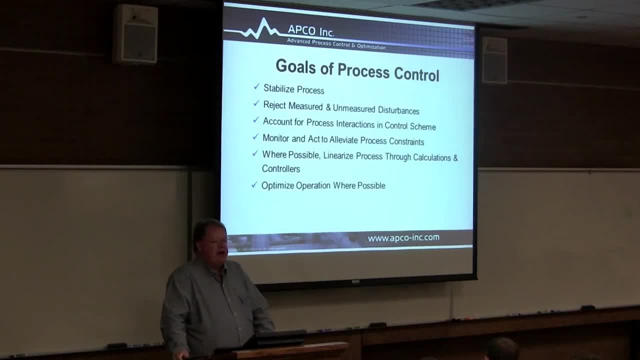 And we're pretty good. okay, That's all it is. If you go out into the plant, it's the same type of thing. Okay, if they open a valve on one side, what happens to pressure on the other side? It's the same type of thing. 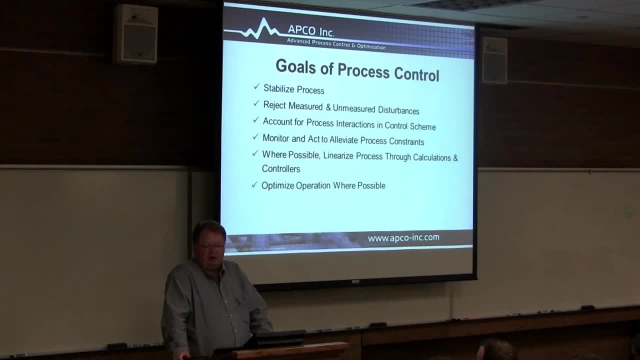 Okay, If they open a valve on one side, what happens to pressure on the other side? It drops. so what happens to the flow on that side? It drops, because pressure's what drives flow. right, Okay, you see. so it's not real complicated, but since we know it, 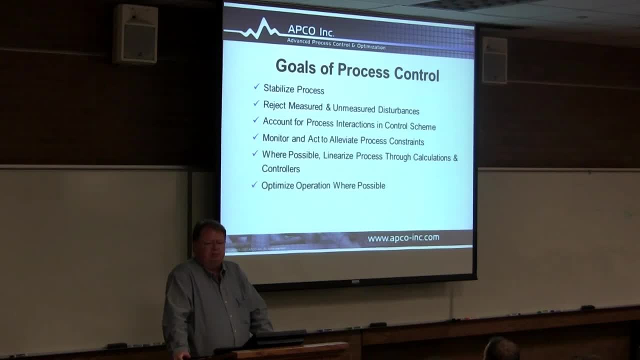 does the computer know those things? No, computers are really dumb, They really are. Computers only know what we program into it. all right, So process control is at least 50%, at least 50%, saying look, I'm a good engineer, process engineer. 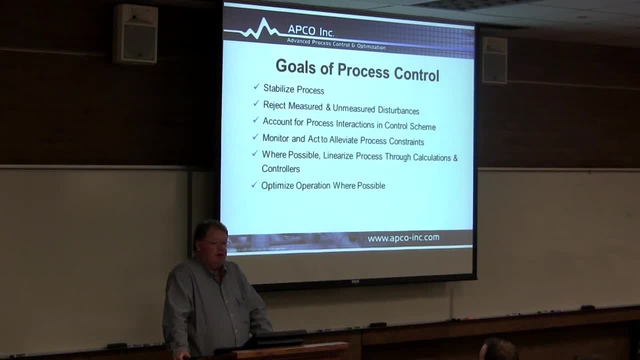 and I'm gonna take what I know about the process and I'm gonna build that into the controls. So does that make any sense to you? So I know, if the pressure drops and the flow drops, maybe I should drop the hot water flow too. 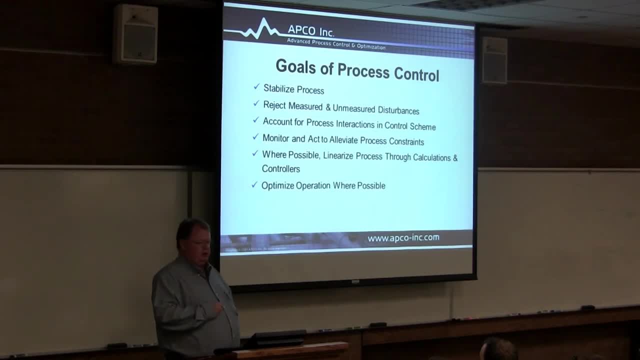 So maybe I should control the ratio of hot and cold water to the shower head. Does that make sense to you? So if I control the ratio of hot and cold water to the shower head when the toilet flushed, would I get a hot water surge? 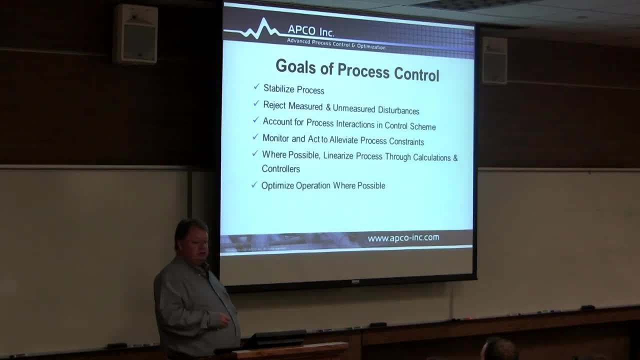 Well, the pressure would drop a little bit, but the water temperature would stay the same, wouldn't it? One of the reasons why we like to reduce variability is because we like to come up almost always the optimal place. The TA is the optimizer, Mr Optimizer there. 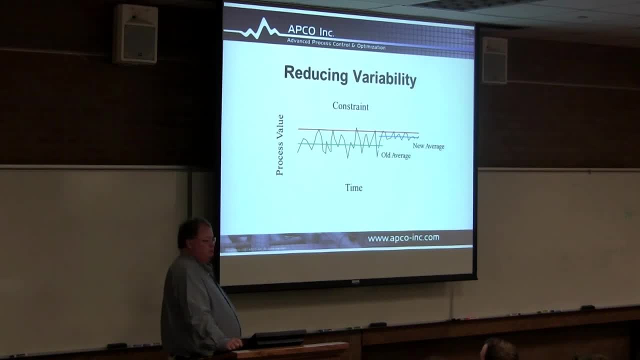 The optimal place to run a plan is almost always at a constraint. Why do I say that? Anyone have any ideas about that? Why is the optimal place almost always to run at a constraint? If I design a tower or a plant, it's: a plant to run at 10,000 barrels a day. They usually want to run more than 10,000 barrels a day in that plant. Why They make more money. They make more money See the capital cost, the cost of the tank, the cost of the pumps. 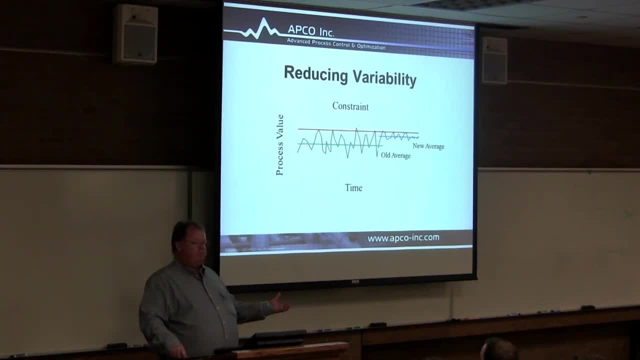 that's a fixed cost, right. But I know for every barrel I put in I'm going to make money on money coming out, right. So how many barrels do I want to push through there? As many as you can. As many as you can, right. 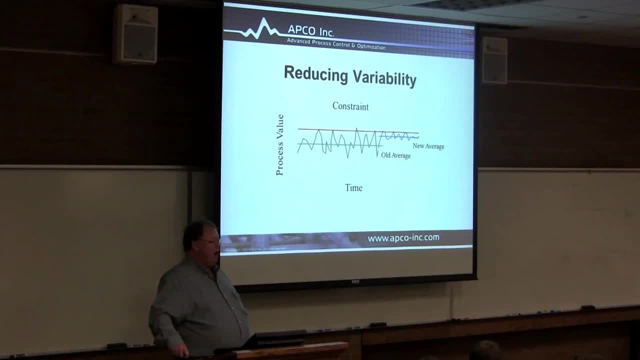 See how that works. It's really quite simple. It's nothing real complicated. You say, hey, I'm going to push as many as I can. Pushing as many as you can means you're going to push that refinery harder and harder and 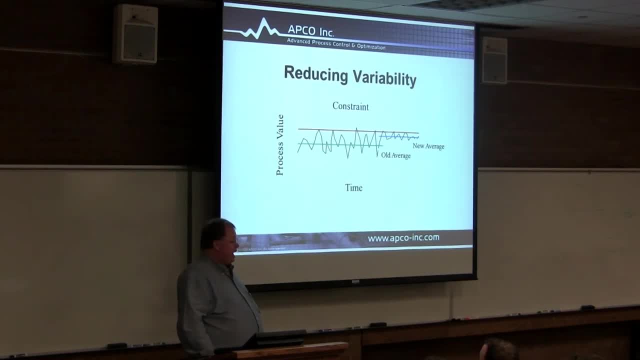 harder. until you do what? Until you come right up to the edge and break it right. You don't want to break it because if you break it it stops. right, If you break the car, it stops. I had a friend. 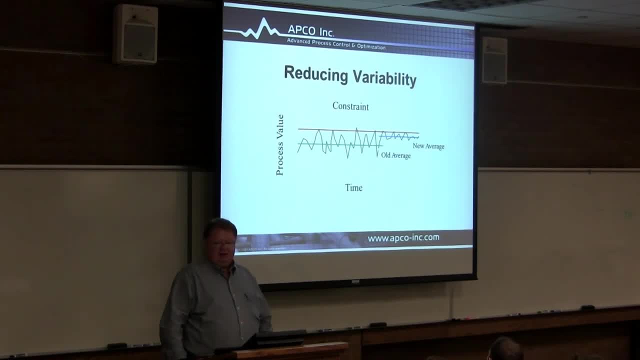 I like motorcycles, I would go out single track in the mountains. I had a friend who bought a KTM 300. He was so proud of that KTM. It was really fast. So he actually bought a KTM 300. He was so proud of that KTM 300. 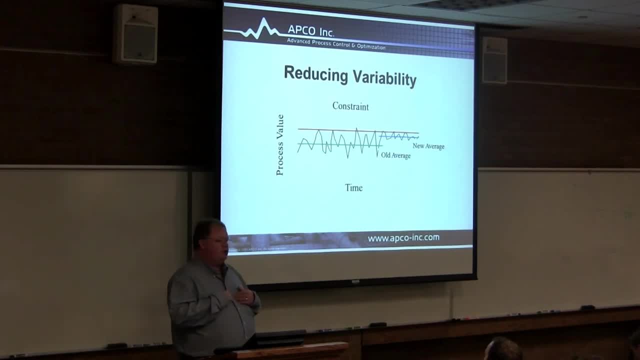 He was so proud of that KTM 300.. He was so proud of that KTM 300. He actually bought a KTM in Miami and he just go riding on that. So he took that KTM. he took it up to 95 miles an hour. 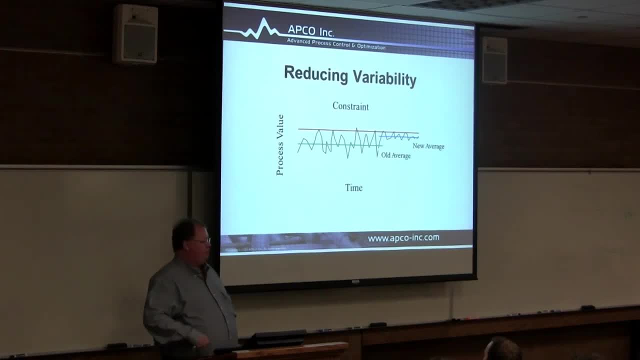 He said, man, he had that baby maxed out, It was doing great. What happened? He blew the engine. Whoops, That went off great. but you know You want to blow the engine, right, You walk on the. 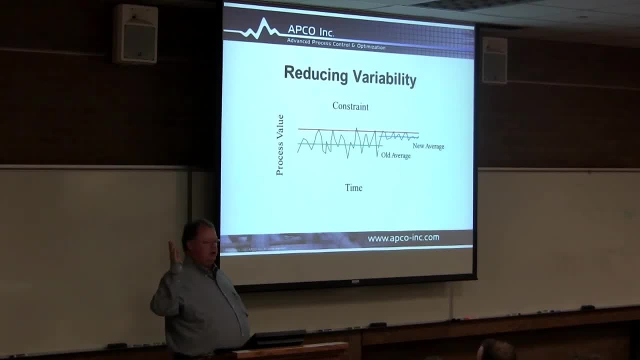 How many of you have ever been out to some cliffs? you know Yellowstone or not Yellowstone, Grand Canyon or wherever? you know Who wants to see how far down it is? Come on, admit it. Aren't we a little bit kind of you? want to see how far down it is? 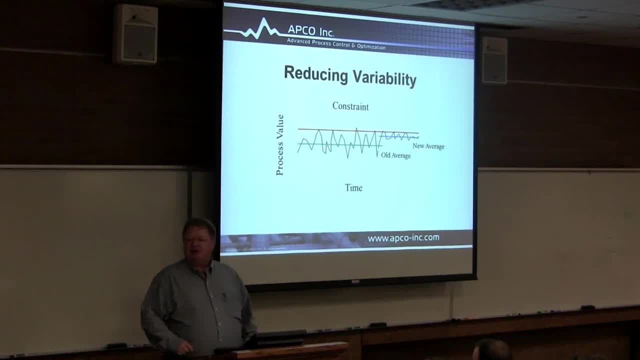 So what do you want to do? You go right, wait a minute. who said crawl, Throw a rock, listen for how long it takes. How many of you crawl over the edge and look over, Or stand over the edge and look over? 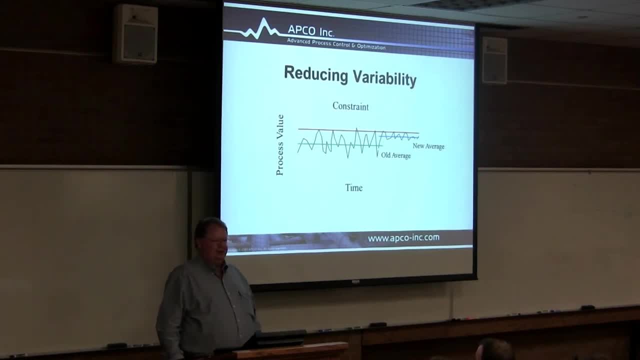 You'd stand up there. You did. I laid down. I laid down: You're hired. Surprise, you're here today. We went down. you know, I threw down on a little soccer thing. we were riding down in the foot clips or whatever, I don't know. 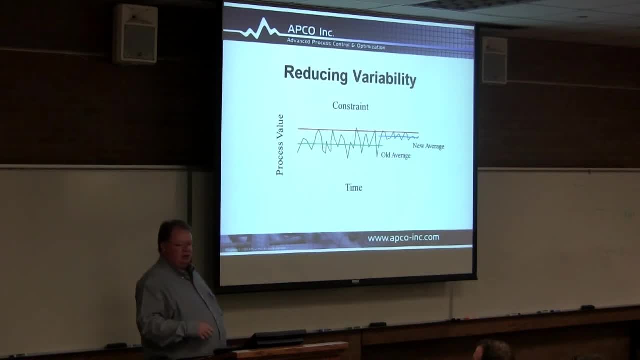 down there. there were some pretty good foot clips down there, so we're riding around and stopped, take a little break. and we just left And I'm like, oh, I'm going to start at the edge and there's this guy that works for me. 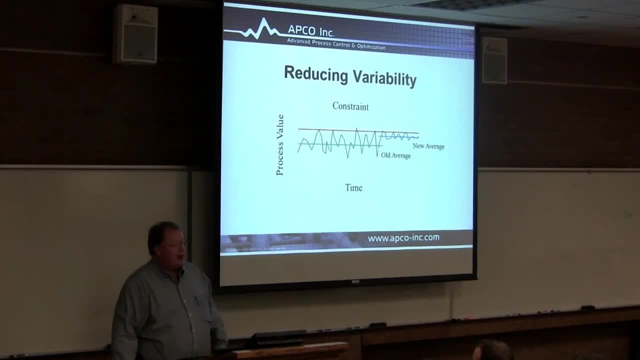 he's standing over there hanging his leg off the edge and I'm just shaking, I'm laid back, I'm like, oh, oh, I just can't walk. you know What is my problem? Can you guys tell me what I'm worried about? 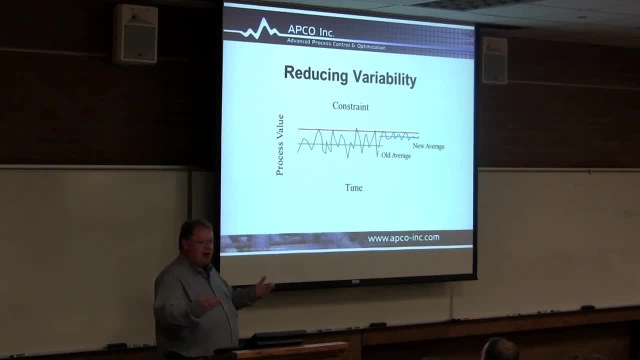 A wind's going to you know blow. there's going to be some kind of disturbance, right, Who knows? he's going to have a kink in his muscle, a glitch, I don't know. he's going to sneeze. 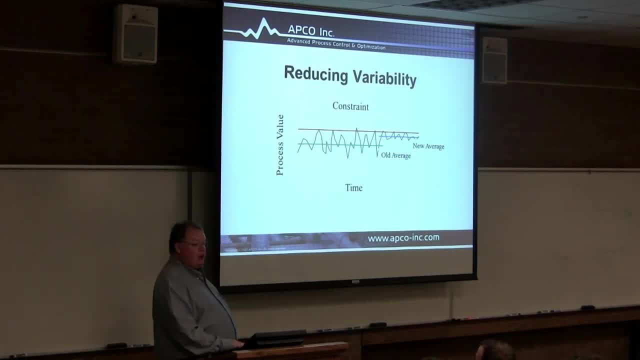 It doesn't take much right. I don't know What happens once he falls off that cliff. There's no turning back At that point. he's like told ya, Just as he hits the bottom. probably That's not the best thing in the world to do. 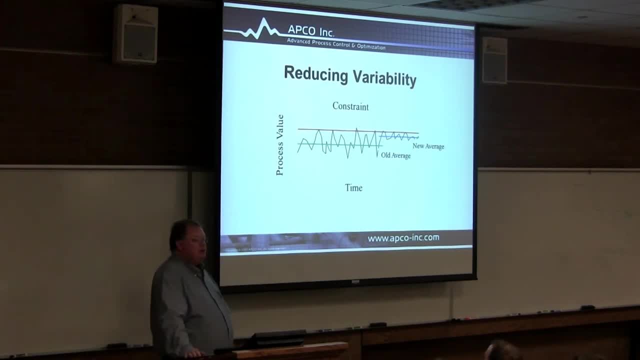 So that's the way processes are Processes. for example, the distillation column, the limitation on distillation column. you guys have had separations. Are you in it right now? Okay, so have you studied distillation columns at all? 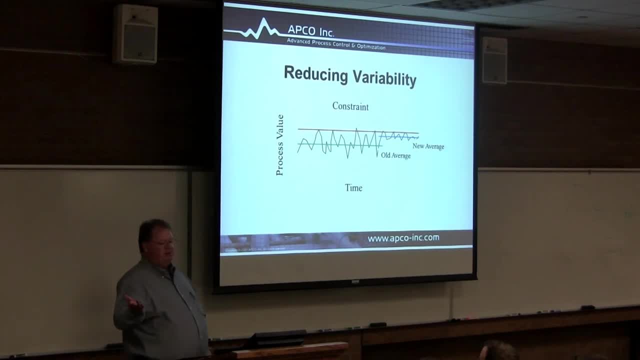 Do you know what flooding is? What is flooding? Liquid, Not water. It's usually liquid. It's not usually water Liquid. It fills between the space, the vapor space, and goes all the way up in that column. okay, 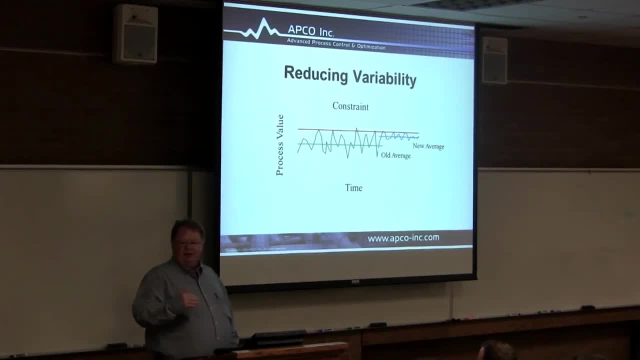 And once you do that, once you flood a column, how much separation do you get? Zero, Zero or close to zero, right, Once you hit that constraint on the distillation column, you're done. You know what you do: Zero. 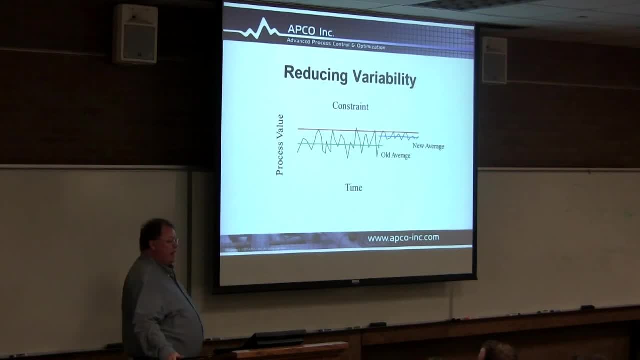 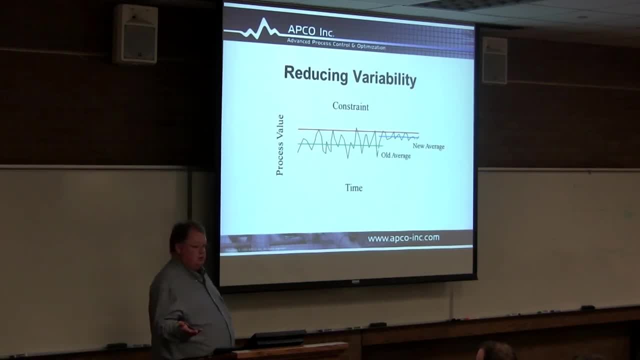 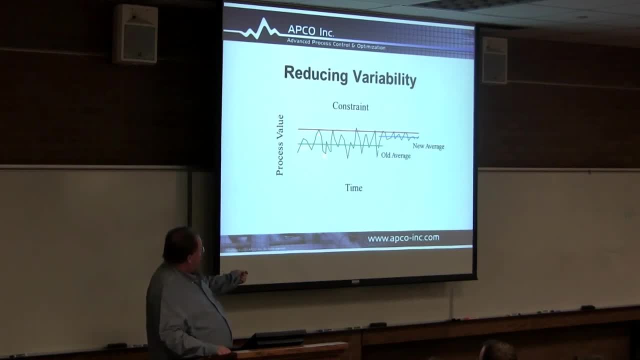 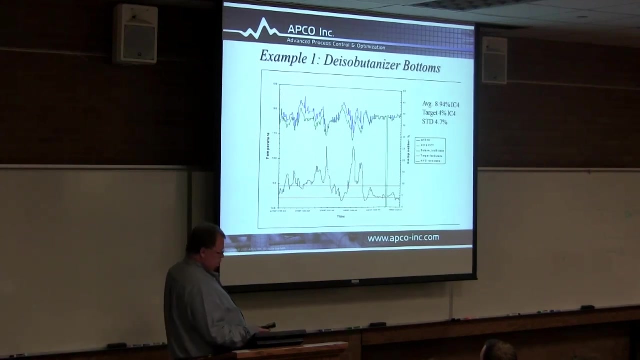 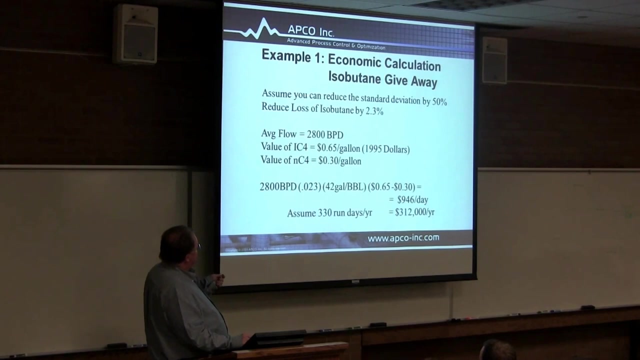 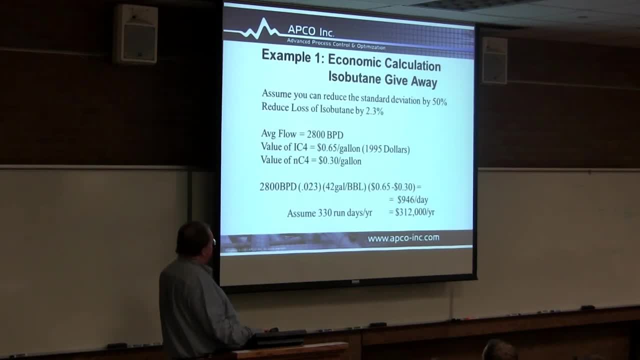 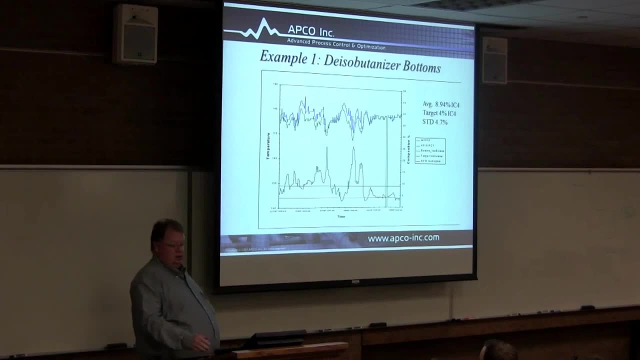 at North Salt Lake and I'll tell you, I'll let you know the entire year on the whole gas. so they said, ok, go ahead and do the project. we don't believe you, it's just computer programming. how much can you really do? what changes control software? so they said, okay, go ahead and do the project. we don't believe you, it's just computed programming. how much can you really do? right, change the control software. so 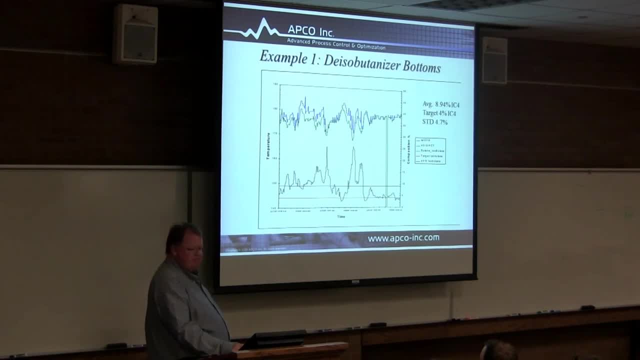 So I estimated I could make them a half a million dollars a year. You know how much I made them: $1.2 million a year Cost them about $100,000.. So if I gave you a dollar and said if you give me a dollar I'll give you $10 at the end of the year, 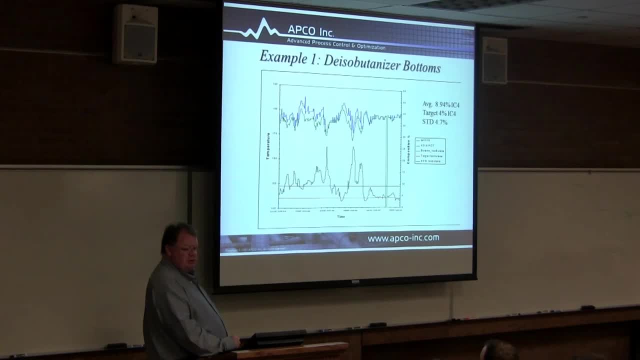 would you do it Pretty good return on investment, isn't it? That's the kind of stuff that process control does, But I'm trying to focus on how your engineering skills can help you work. How many of you in here know about the Antoine equation? 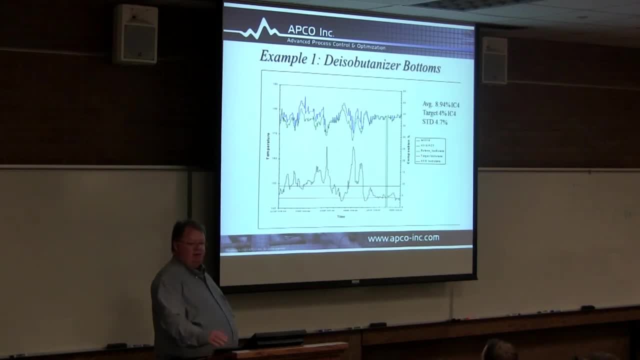 You've just heard of the Antoine equation. Every hand in the place should go up, right? You learned about that in material and energy balances. What did the Antoine equation do? Vapor pressure. So the Antoine equation can give us information about varying pressures in a distillation column. 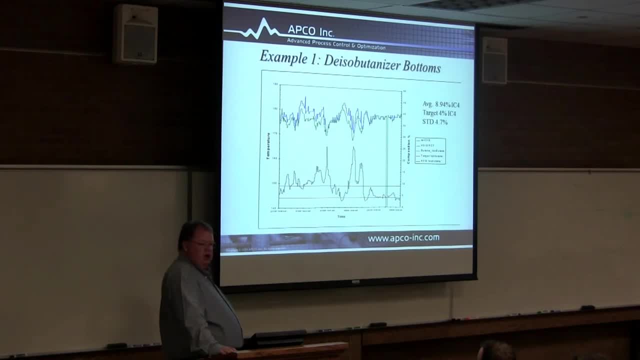 So if I increase the pressure or decrease the pressure in a distillation column, the separation changes. Do you know that? So the problem is that they want to control the pressure of the distillation column. So they want to control the pressure of the distillation column. 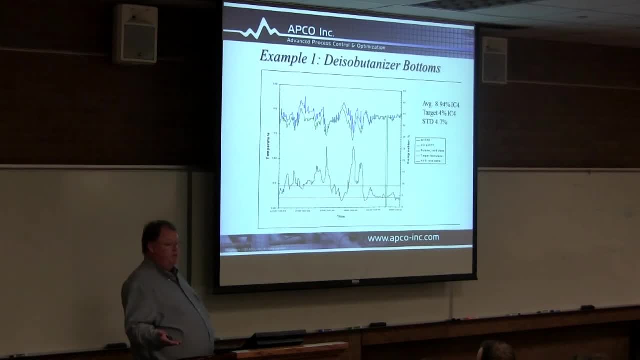 So they want to control the temperature, to control the separation, But the pressure is jumping all over the place. That's a disturbance, right? See how that works. So the pressure is a disturbance to the separation, isn't it? So we did what we call pressure compensating. 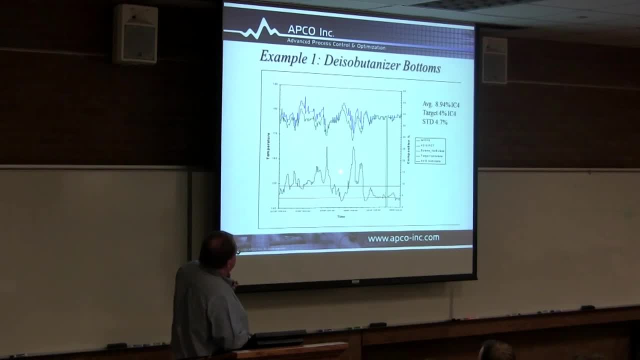 So you see, this black line in the bottom is the analyzer. That's isobutane. The bottom line is the amount of isobutane going out. the bottom That's how much they want to go out. That's based on a steady state analysis. by the way, 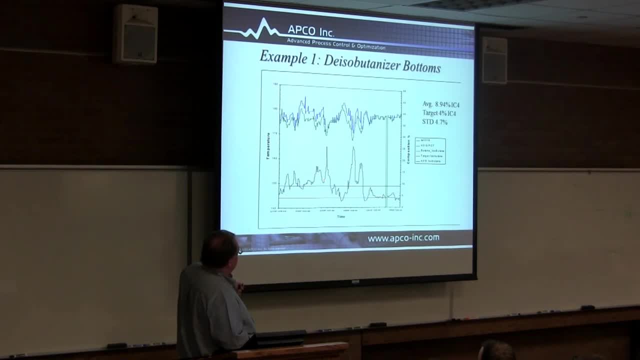 This is the actual data. Each one of these little bumps you see is like 40 minutes or something like that. So this is probably a few weeks' data, or even more. This is the temperature of the column, So there's two different things here. 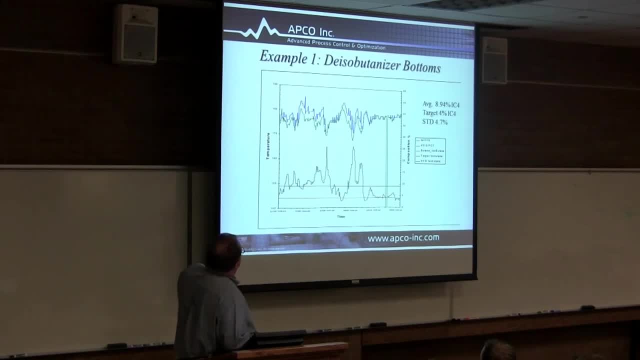 One of them is: the blue is the actual temperature, The green is the pressure compensated temperature. So what happened in this column? up there they have air cooling. We're not by the ocean, The ocean they always use. We're near the ocean. 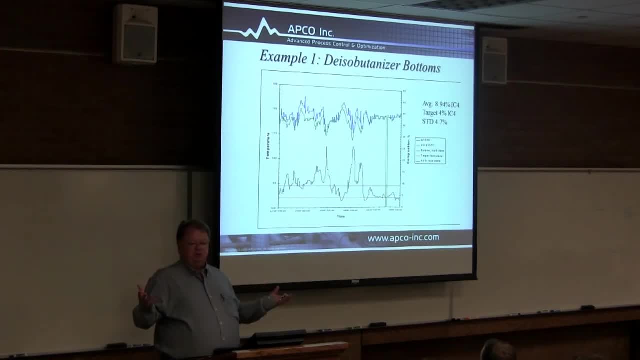 Near the ocean or water, they always use liquid-liquid heat exchangers for the most part to do their cooling. They've got a lot of cooling water there, right, But up here in this dry, arid desert, we have a lot of air. 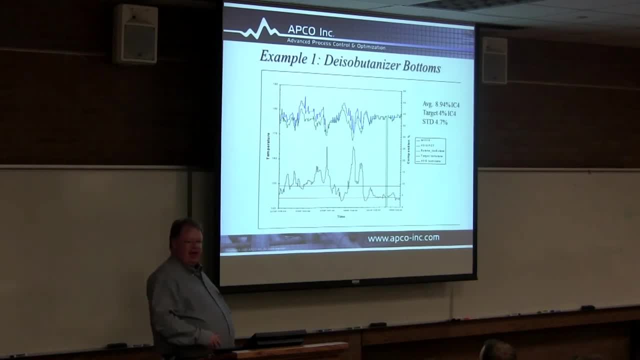 So we use what they call big-bang heat exchangers. You've probably seen those in the lab. Those are very simple compared to what they use in industry, But they use these box exchangers. What happens on the hottest days in the summer? 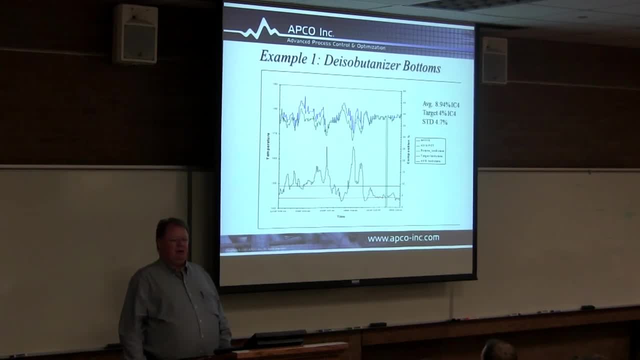 It's hot And they get enough cooling. No, Because they don't get enough cooling. Pressure goes up. right, PV equal NRT. Temperature goes up, Pressure goes up, Okay, So here's this green line. here The blue line is the actual temperature. 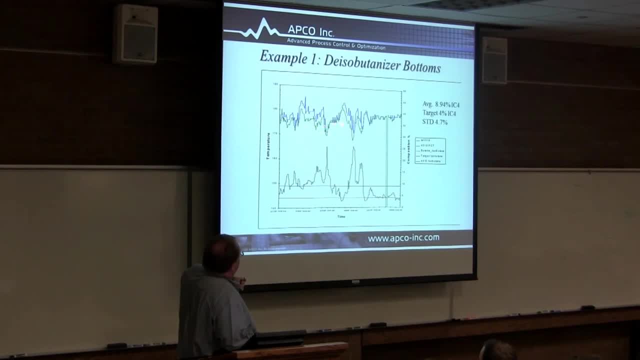 The green line is the pressure compensated temperature. So you see, for example, in this section right here, you see that blue line bouncing all over heck and back. Okay, You see, the green line has that. It's fairly smooth. Look down here at the analyzer. 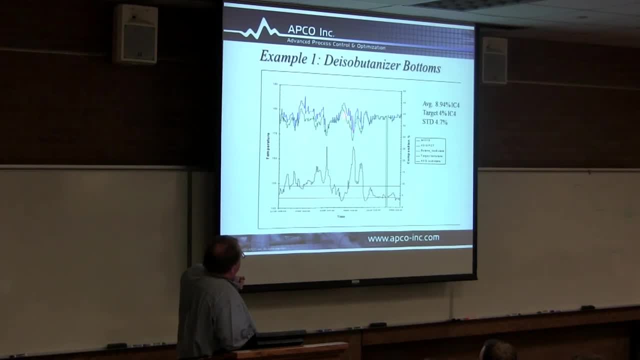 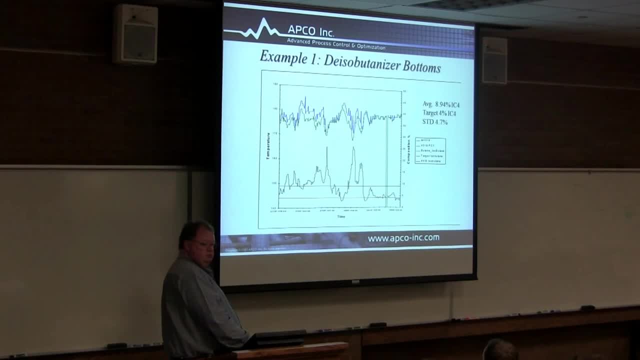 ECT, ECT, ECT, ECT, ECT, ECT, ECT. It's a simple engineering calculation. So if I control the pressure compensated temperature and I use that as an approximation for composition rather than the actual temperature, which one's gonna do better. 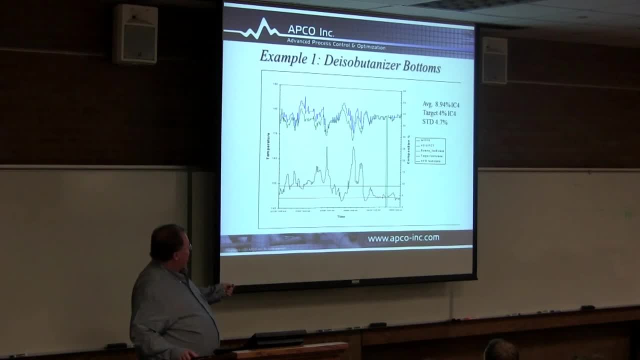 ECT, ECT. So here I turn on my controls And I reduce my standard deviation by 50%. So here's the place where I lock my analyzer. You see that. So you think I made him the money that I said I was going to make him. 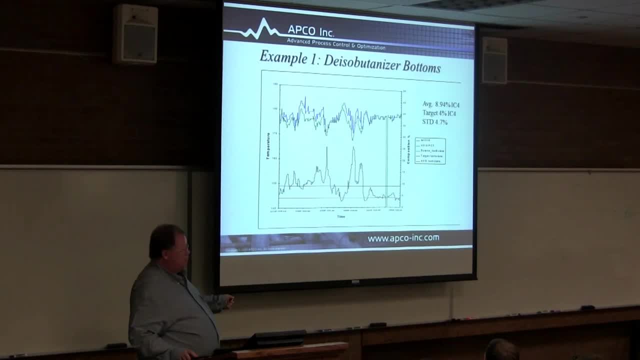 So that's the example of before and after doing some engineering calculations and doing some very simple controls. Improving the controls. Does that make any sense to you? That's pretty good money, isn't it? That's not bad. Would that pay your salary? 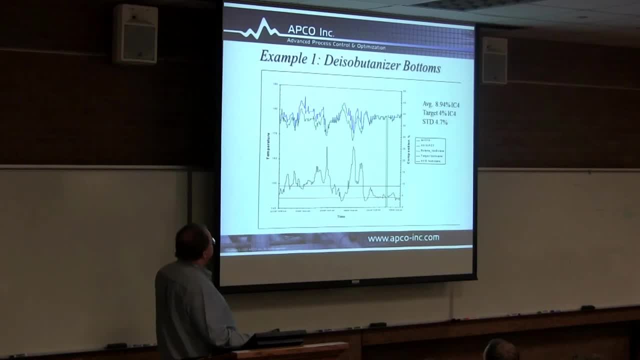 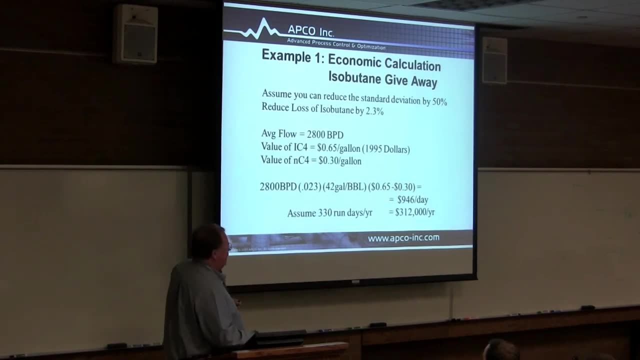 for a year? It probably would. It would for multiple years if it were working. for me It would be like a decade. Sorry, No, that's not true. I have to try to beat the stereotype right. Here's another one for you. I did one down. 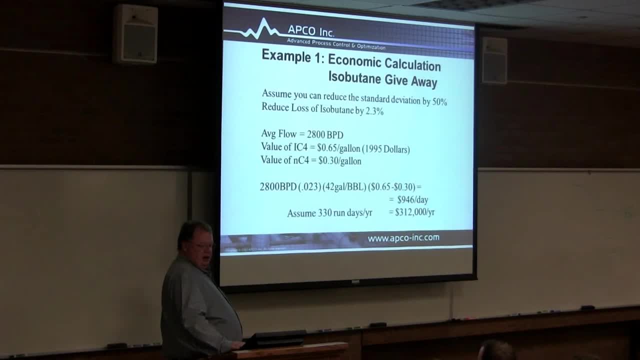 at a sweetie refinery down in Texas We did a propylene splitter. You guys know what propylene is. Yes, What's propylene used for Polyplastics, Polypropylene Plastics- Okay, Valued it, Valued the stuff. This is a $995.. 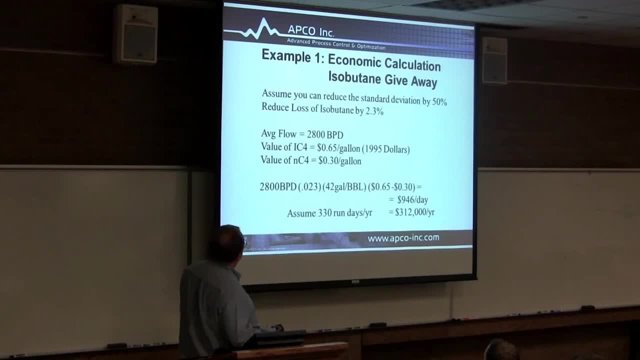 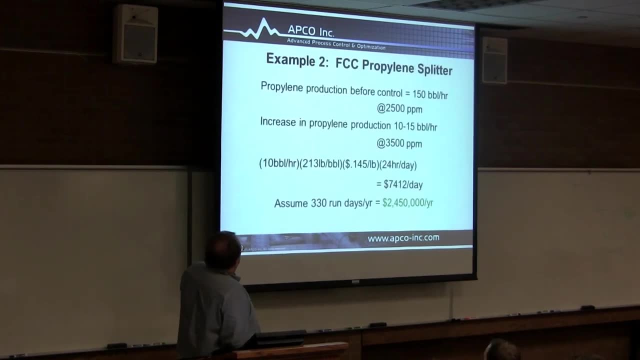 Oh, that's the same one. Next slide, Come on, Come on. Before it was 150 barrels and 2500 parts per million. Increase in propylene production by 550 barrels per hour. 3500 parts per million, 10 barrels times 213. pounds per barrel. 14.5 cents per pound, 24 hours a day. $7,412 a day: 330 run days a year: $2.45 million. I didn't think you'd see that When we started to work. 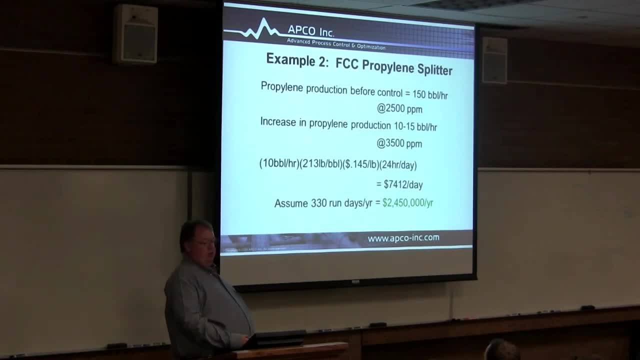 the Big West refinery. they were barely profitable But because of the process control and because they get added processes that made them money, they're now an extremely profitable refinery On the orders of multiple hundreds of billions of dollars a year of propylene. 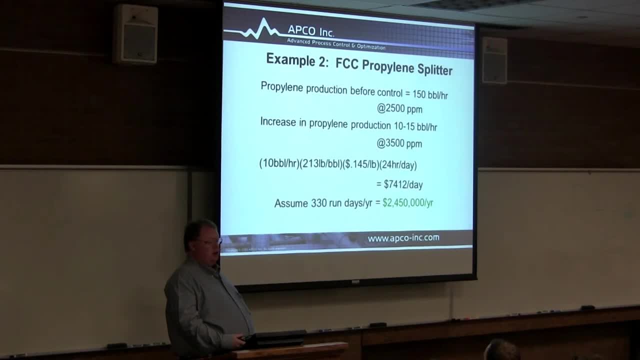 So if you can walk in and you can say, hey, look, I can do some things for you, you're going to be a hero. Okay, Do they come to you first, or do you go to them and say, hey, I can make you some money? 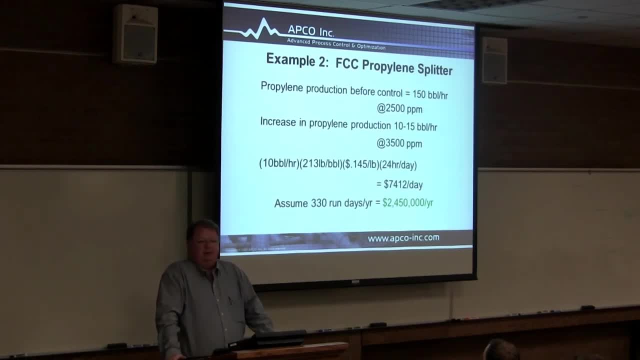 I've been in business for some time now, but I'm not a very good businessman. Can I tell you something? I'm an engineer. I'm not a good businessman. I'm actually not a bad businessman, but I don't do some of the things that are good. 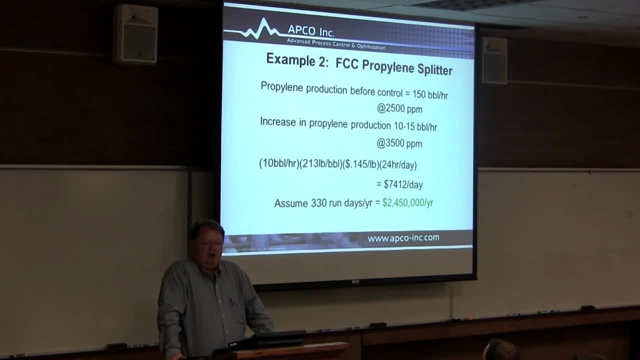 I don't go out and knock on doors. It's just not in my nature. I'm a pretty outgoing guy, but I find it hard to knock on someone's door and say, hey, look what I've got to show you. So the way I do it is, they call me up. 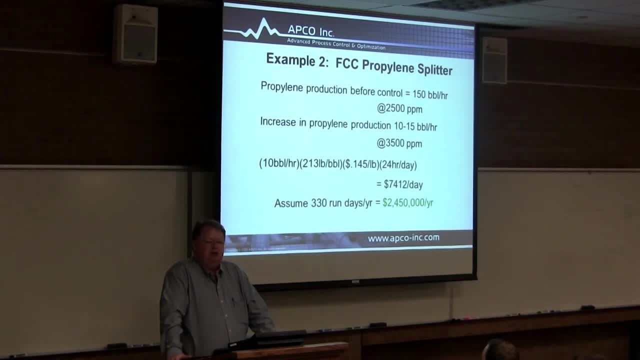 with a problem, I go in and help them solve the problem and I educate them. So a big part of what we do in process control- and what you'll do as engineers, I guarantee you, is education. There's a salesman component in every. 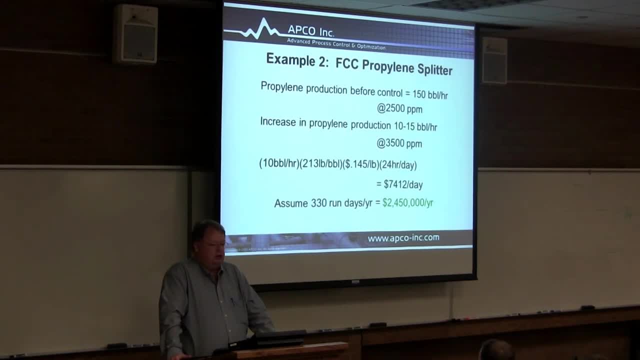 engineer's job, Every single one. I don't care where you work or what you do. You're going to have ideas. You're going to have things you think you want to get done. You're going to have to sell someone on those ideas. Okay, You're going to have to help them to understand that it's worth. 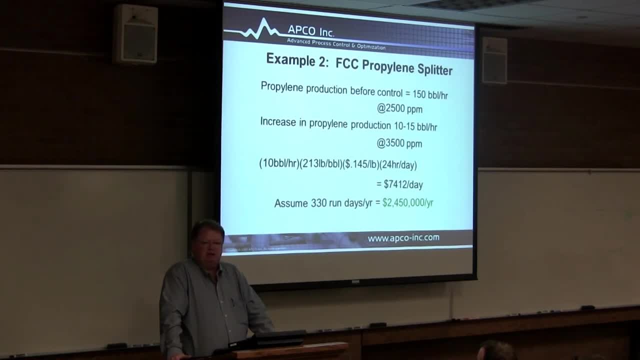 their, while Economics is almost always the best way of doing that. There's other safety and other things like that that can do it, But economics is the best way to do that. So, thinking about things in terms of economics and how to do the economic analysis to justify So, on this one I made some 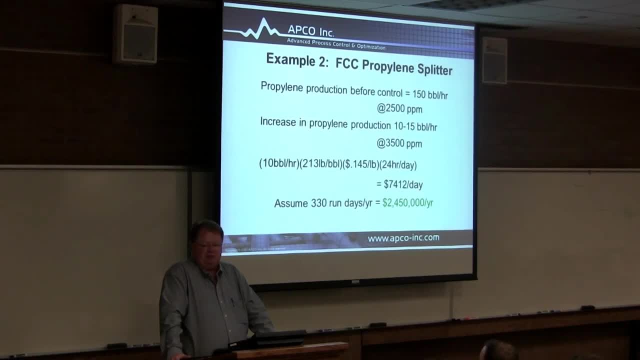 assumptions, didn't I? I assumed I'd be able to reduce their standard deviation by 50%. I learned that from experience. Is that hard to do? No, Not for me, It's trivial. If I had gone in there and said: I'll reduce your standard deviation by 90%, what do you think? 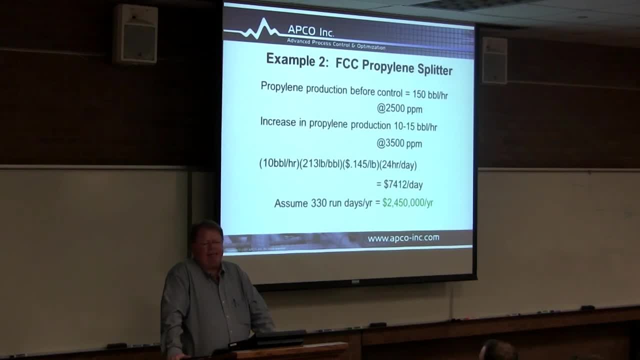 they would have said: Black, oh, yeah, right, black magic, Yeah, what are you going to do? Right, we're better than that. But if you look at it, I probably reduced it by 80-90%. So you have to be realistic. 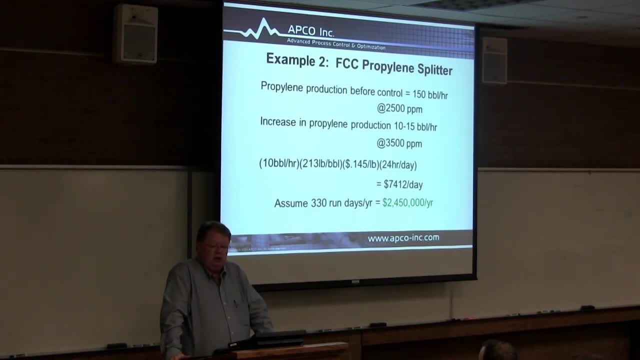 My goal is to always give good estimates of what I do, conservative estimates. So when I told these guys I was going to make them $500,000 a year, and I made them $1.42 million a year, what do you think they did? 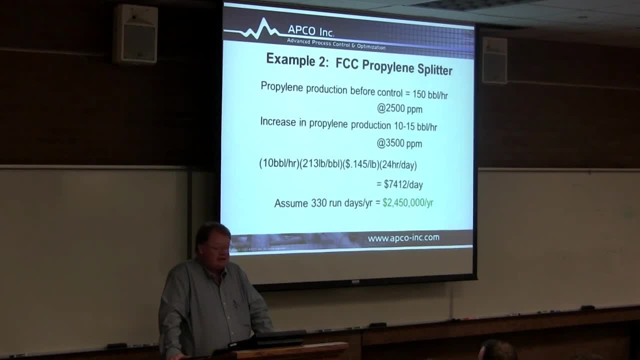 They came back and said, wow, that's on our gas plan. That's not supposed to make any money. What would you do if you did the rest of the plan? So we've done all the process control for the last 15 years. So my way of doing. 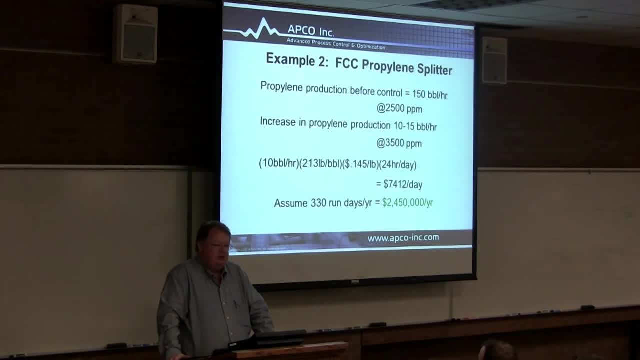 business is to not go in there and try to make somebody pay through the nose. I did come to this company after the first job and I said I'll tell you what I'll do. I'll do the rest of your plan and it won't cost you a nickel. 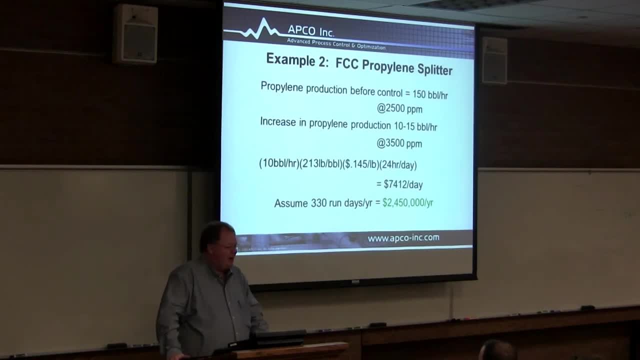 Now, how's that sound? Sounds like a better businessman. Sounds like the guy selling you a water softener or something. to me, What I'll do is I'll take 10% of your incremental benefits, Just 10%. Just like this one we'll pull. 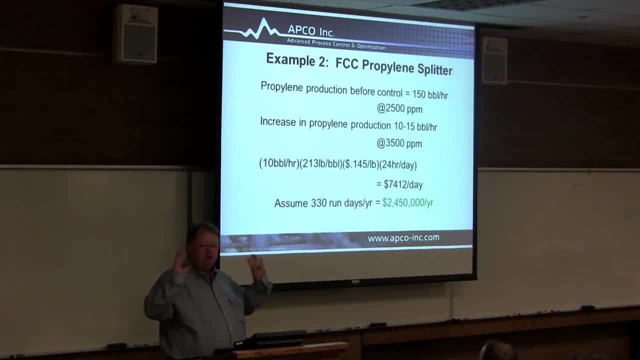 a bunch of data before we'll pull a bunch of data. after we'll run it for a year, we'll see what we make The incremental benefit. I'll only get 10% of that. 90% of that will be. 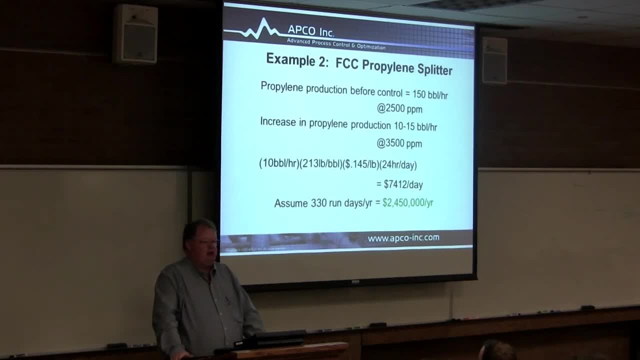 yours Just 10%. 10% per year for the next 5 years. So if I did 10% per year for that one for the next 5 years, I would have made $120,000 a year for 5 years. I would have done alright, wouldn't I? 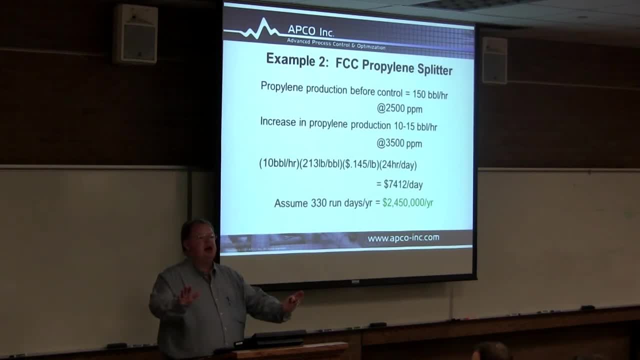 You know what the refinery manager told me? Don't worry about it, just tell us what your rate is and we'll pay whatever it is. And we did the rest of the plan that way. He didn't want to pay me a percentage because the dollars 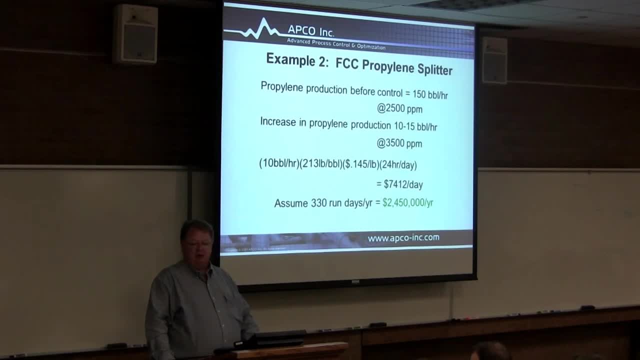 are big. It's like getting into other things like a cat cracker and a reformer appellation and things like that. That's lots of millions of dollars a year in Jamaica. So the answer is: I don't knock on doors. They usually come to me. One of the 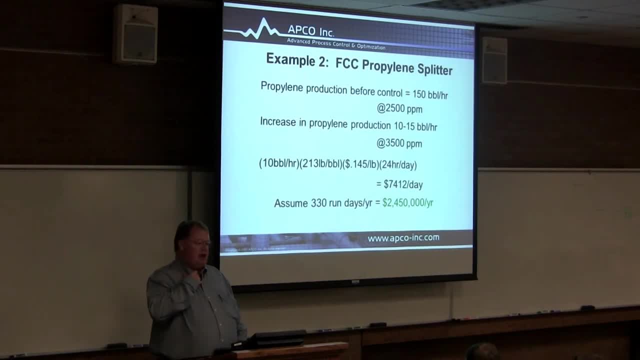 things I'll tell you about business is my business is not what I anticipated it would be. When I started my business I came back from Setpoint. I was Super Mister Advanced Control. I was a software development manager for this worldwide company. I was all over the world doing this stuff. I had lots of contacts in industry. 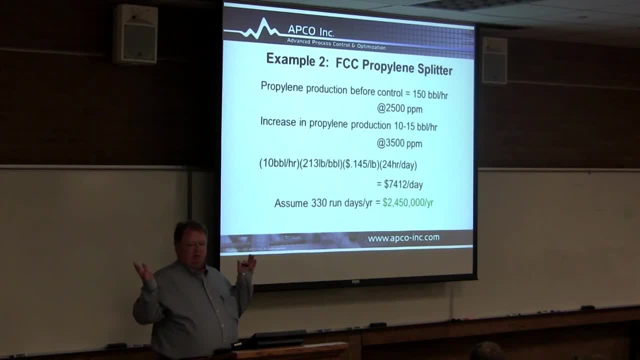 and I came back and I thought, wow, I'm going to do work in the heavy industries, Chemical plants, I'm going to make my millions and go home and be happy. Well, the first thing I'm out there working on is the Big West Refinery and 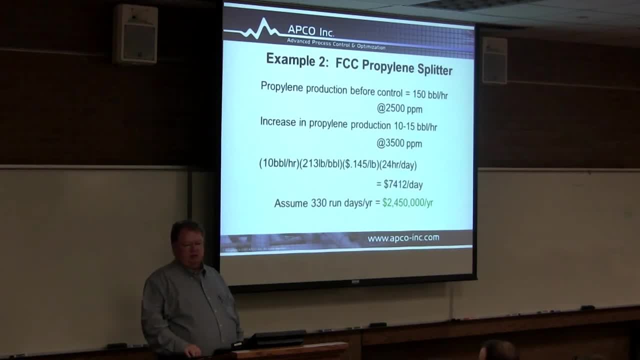 the next thing I know: Central Utah Water. Do you know who they are? Central Utah Water controls most of the lakes and stuff. They control the water flow for most of northern Utah, Provo River, all the other rivers, Jordan, Owl, Strawberry, Starvation. 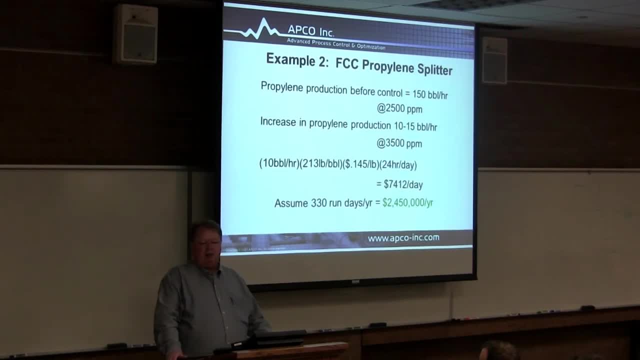 blah, blah blah. They have three water treatment plants. They come to me and they say we've got a problem. We've got this company we hired out of New York and they put in a system called SIFAR and it's not working and we had a big problem the other day. The problem: 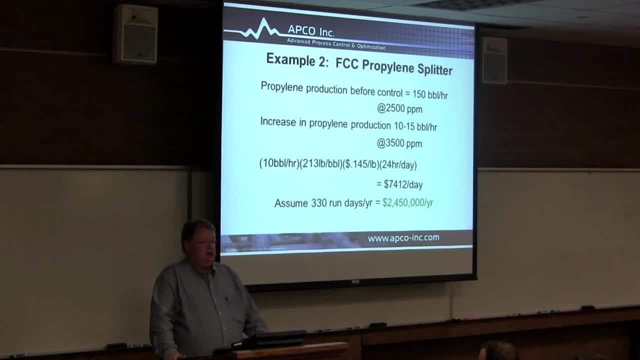 with the Jordan Owl Dam. You guys know what the Jordan Owl Dam is right, So you know what the problem was. What's the worst thing that could happen to the Jordan Owl Dam? It could break. What's the second worst thing that could happen to the Jordan Owl Dam? 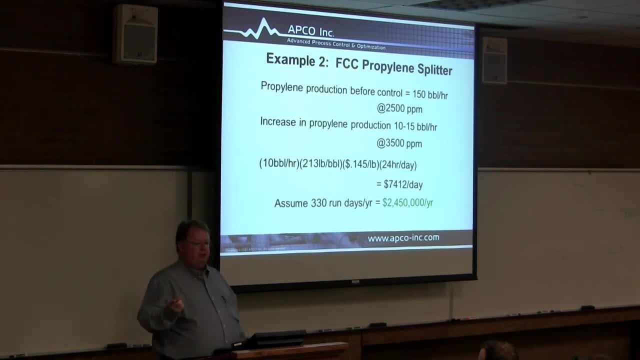 Flood gates would open. The gates would open, right. What would happen if the gates opened? The river would be underwater, right. That would be bad, wouldn't it? I would contend that that's not quite as bad as what happened to them. 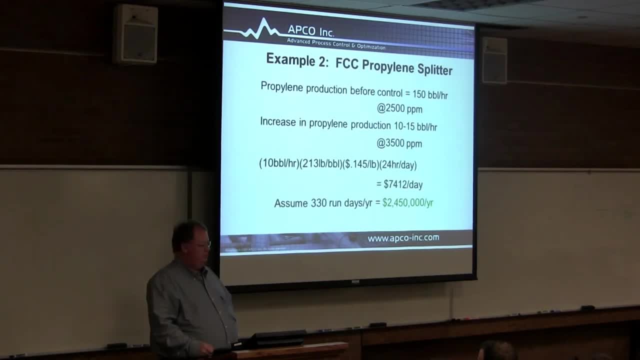 The gates closed all the way. What happens if the gates close all the way? Huh, Provo River dries up. Oops, I'm not good, but that's bad. You know, the only thing worse than killing people is killing fish. 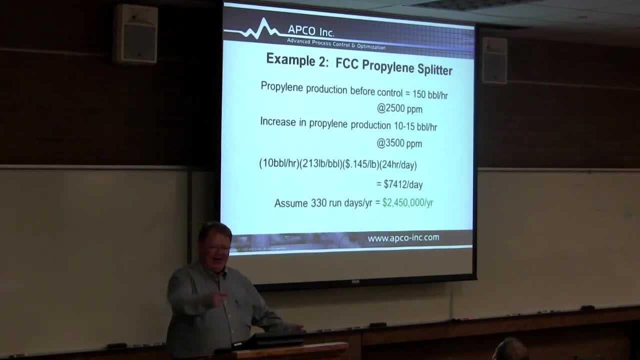 Come on, We're the fishermen. He knows what I'm talking about. Alright, I mean you flood a hole or two, you can pump the water out, You kill fish. That's a decade or more before you recover from that. 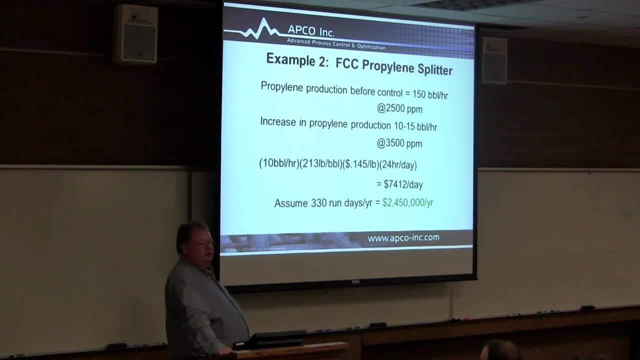 That's a long time. That's bad. So the gates slammed on the Jordan Owl Reservoir, okay. So we went up there and we put in a bunch of stuff that we do all the time in the Kimmelton industry, The refining industry, A bunch of safeguards. right, Can I have a valve slam open? 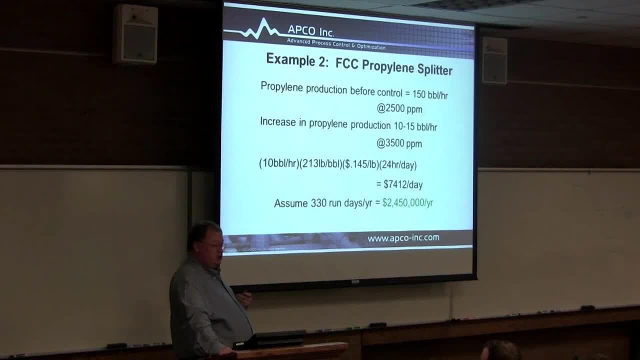 or shut in a refinery. If I do, there's a good chance somebody will die. That's not good. Happens all the time. That's not good, right, Okay, So we already built in safeguards, Lots of safeguards. We're very good at it, Very, very good at it. 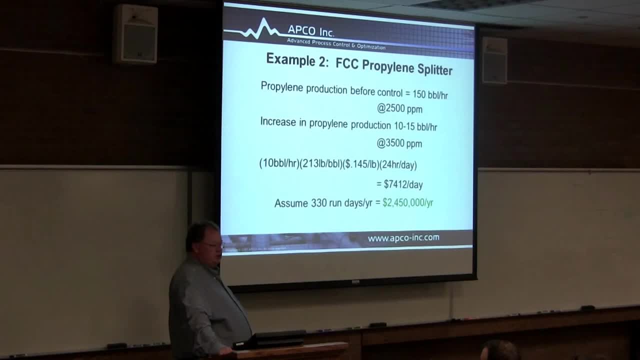 So they come to us and they say: we want you to re-tool our system. How much has it been cost? I say, okay, man, I think about $200,000.. I just go up there. It popped, It, popped that out. 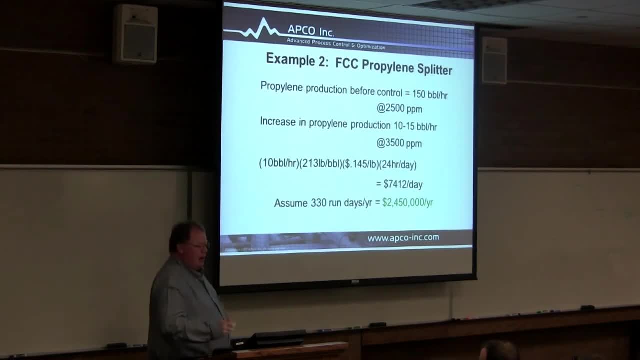 That's a salesman. I don't have a dog. I react to the calculation. I'm not quite reactivated Anyway, so we did it. They had a guy working there. He just started the day that we started working there And he did most of the panel work. Changing power supply. 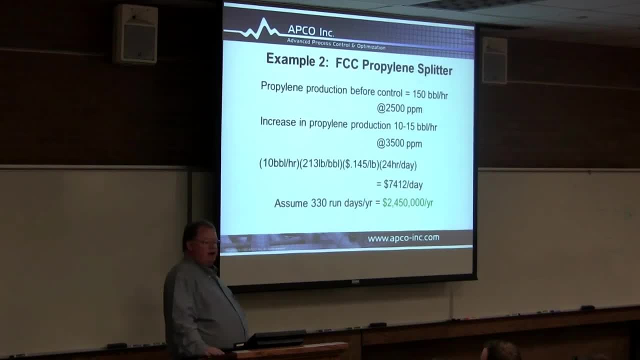 so we went back and said: look, we've got like $100,000.. The project's done, You've got $100,000 left. Whoa, whoa, whoa. wait a minute, What do you mean? we've got $100,000?. 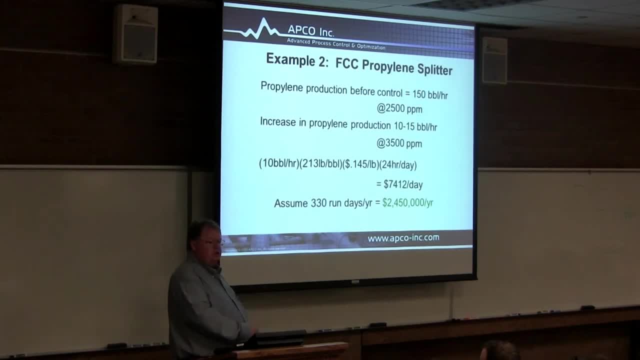 We're done. Your guy did a lot of the work. You told us it would be this much. You haven't charged us that much. Send us a bill. No one comes to us and says, no, we don't want your money. 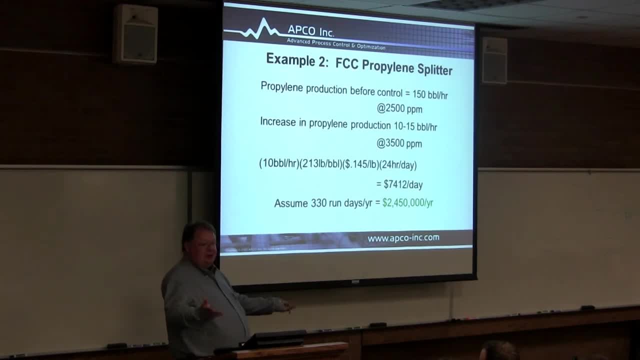 We said, well, your guy's good, He helped us. What do you want us to do? They said, well, we've got a wish list of things that we wish our system did. They said, well, give us the wish list, We'll work on the wish list. 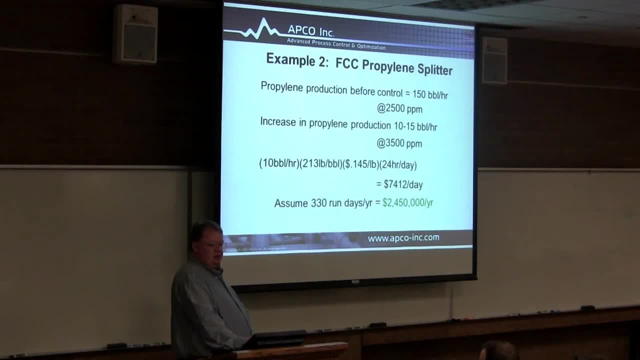 They said: well, give us the wish list, We'll work on the wish list until we run out of money. We said, great, We got almost all the way through the wish list, And that was 12 years ago. We were doing all the control work. 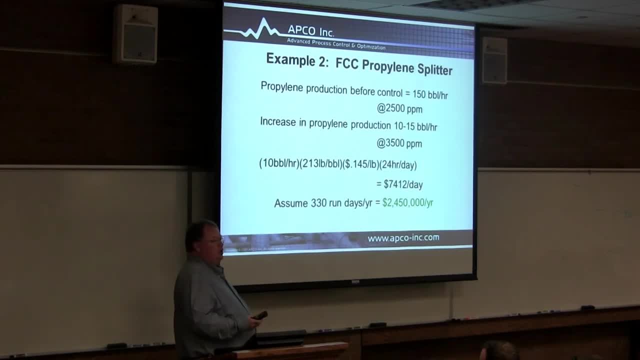 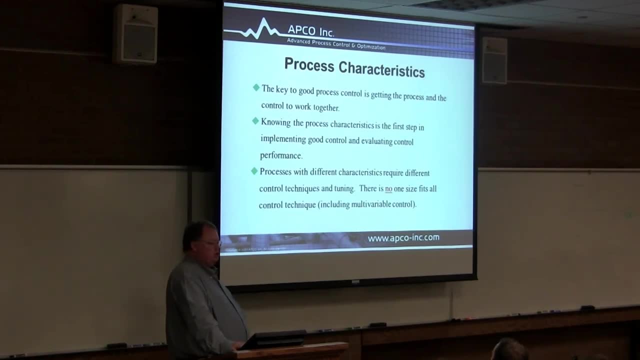 We are, So being honest. one of the things about being who we are is being honest about your work is good, So you don't need to try to cheat people. Just because you can doesn't mean you shouldn't. So I treat my employees. 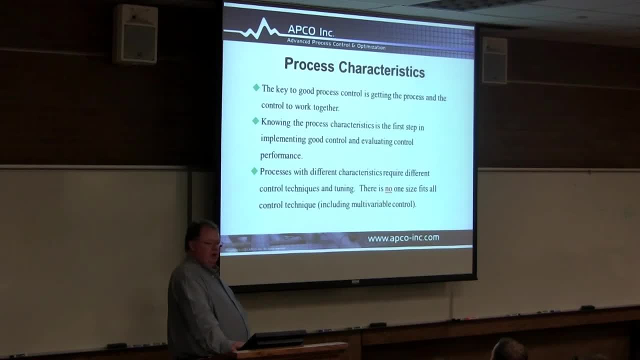 and my clients, everybody the same way. I'm very, very open and very direct with them, which is a good thing on everybody's side. If my employee's not doing well, I'll tell him he's not doing well. I'll tell him why he's not doing well. 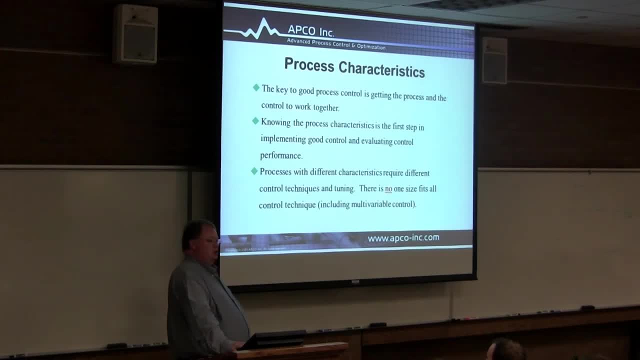 We'll do what we can to help him get better. Same thing with the client. I don't go to my clients and say: don't pay attention to what we're doing because this is top secret, proprietary. I'd have to shoot you if you saw. That's not my approach. My approach is: 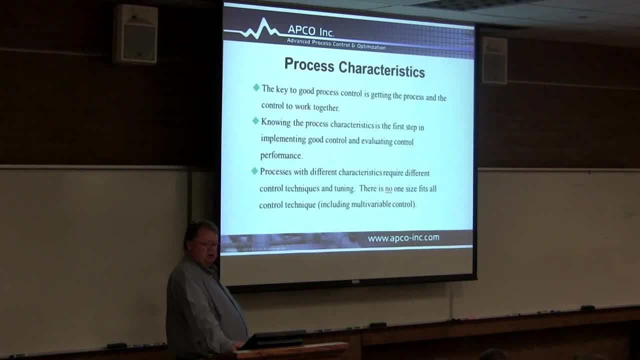 yeah, have someone stare over our shoulder. Anything you guys can learn is great. It's your system. You want to know as much as you can about it. The key to good process control is getting the process and the control to work together. 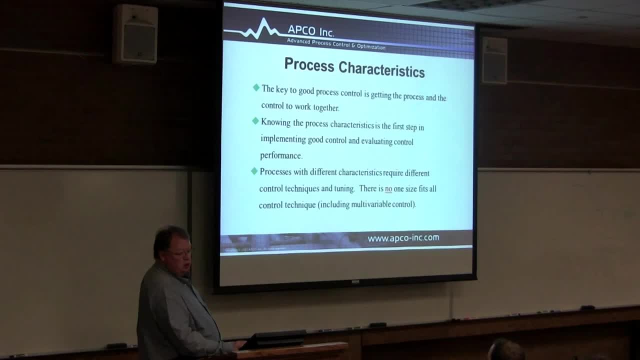 Understanding the process is what engineers do. If it's a matter of saying, hey, it goes up, I'm going to open the valve. and it goes up, it goes down, I'm going to close the valve. I can train a monkey to do that. 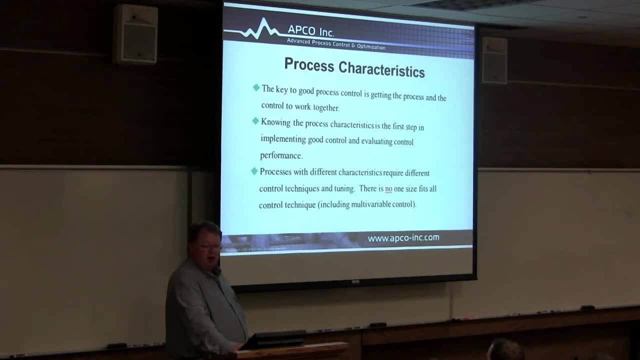 I don't need an engineer. I need an engineer because he understands the process. Knowing the process characteristics is the first step in getting control and evaluating control performance. Processes with different characteristics require different control techniques. No one-size-fits-all control technique including multi-variable control. 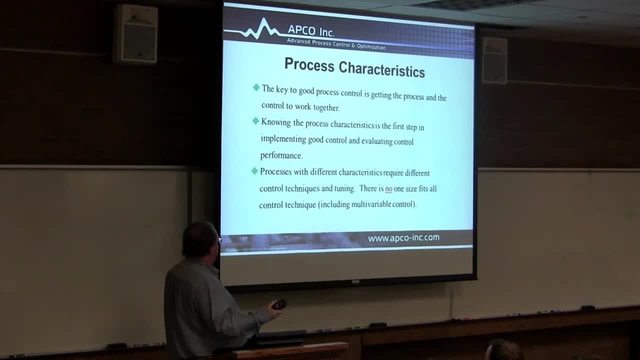 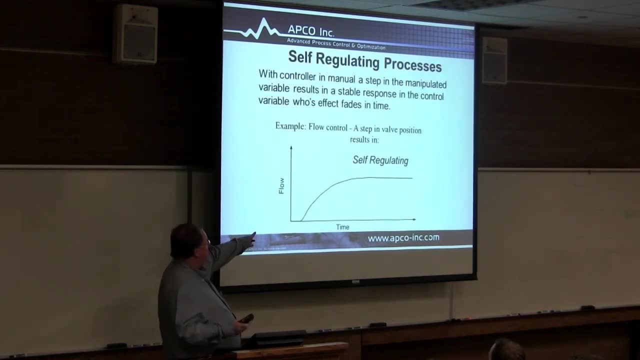 seems to be considered the solution to all control problems. I'm going to go through just a little simple example. We're almost out of time. Self-regulating process. This is the two most important things you need to know about process control- Two most important process. 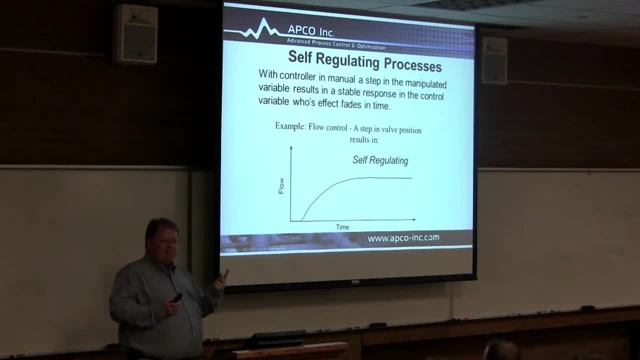 characteristics I'm going to give to you right now. If you pay attention to this next five minutes, you're going to be a superstar. Whenever I go into a refinery or a chemical plant- almost anywhere- most of the problem is they're all doing. 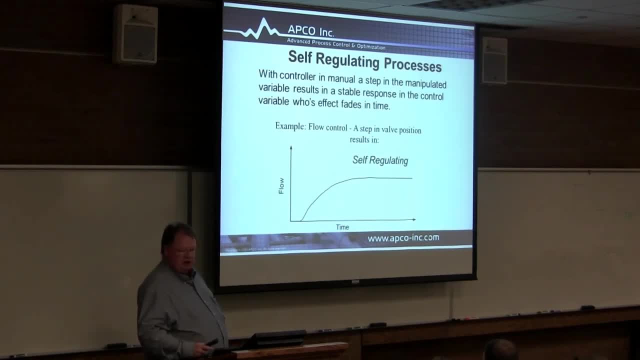 PID control. It's the standard 90-95% of control out. there is PID control And they're trying to use PID control on everything And that's fine. For the most part it works pretty well. But you have to understand. 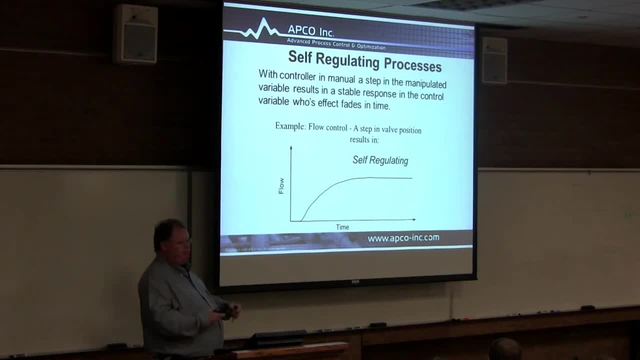 what you're controlling Is the process, self-regulating. What I mean by self-regulating control is, if I open a water valve a little bit, what happens to the flow rate? It increases and stabilizes out at a new value If I open it a little. 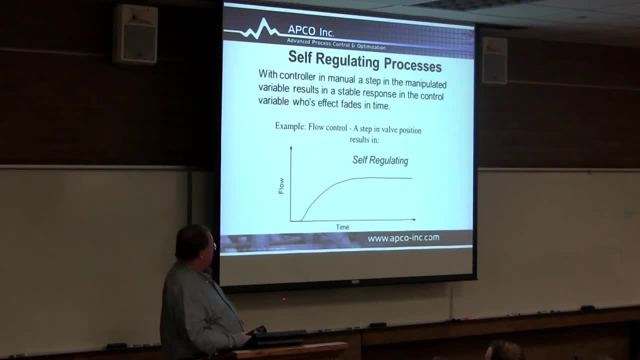 more, it increases and stabilizes out at a new value. Just like that. That's self-regulating. If I increase the heat to the bottom of a distillation column, the temperature goes up, stabilizes out at a new temperature. Does that make sense? 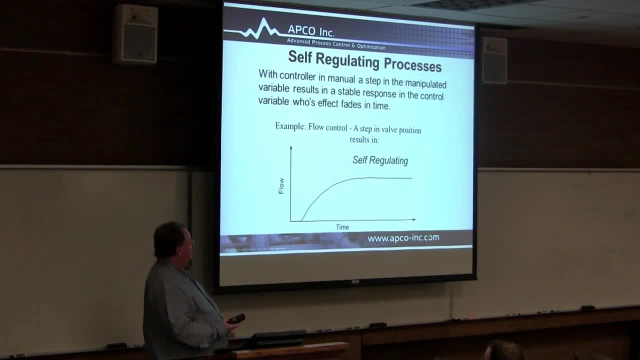 It's called a self-regulating process. In a self-regulating process you use P, proportional, integral and maybe derivative. if it's got a long lag time, But certainly PID control, You have to have the integral or you've got steady-state offset. 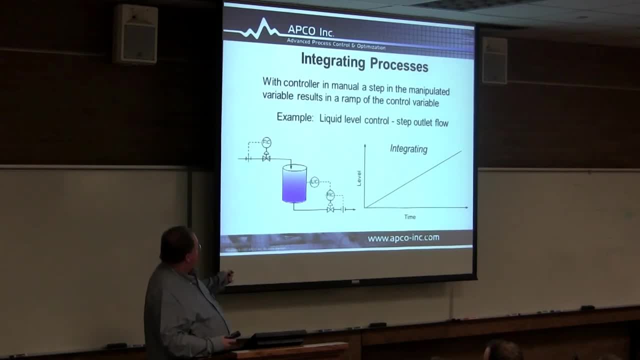 In an integrating process. I make a change. Let's say that this is my thing and I make level loops open. I make a change in my outlet flow. Let's say, I increase my outlet flow. What's going to happen to my level? 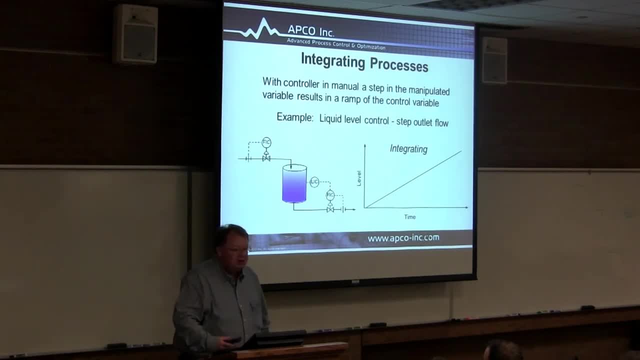 It's going to go down. How long is it going to go down? Forever, Until it runs empty? Or, if I reduce the outlet flow, how much is it going to go up Until? what Do you see the difference in the reaction? 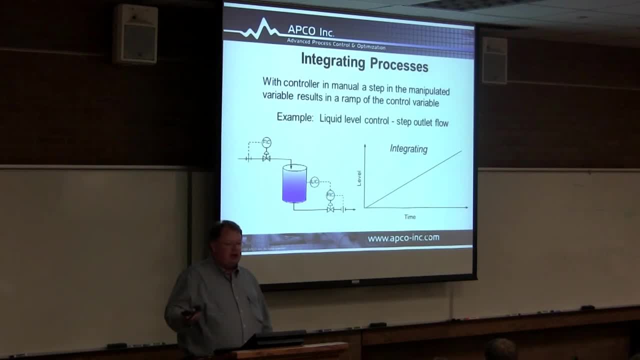 So for an open-loop step, one of them is self-regulating, the other one is integrating. In this particular one, if you have an integrating process, you use no integral control, None. Alright, now you guys can go out and save the world. That little technique probably. 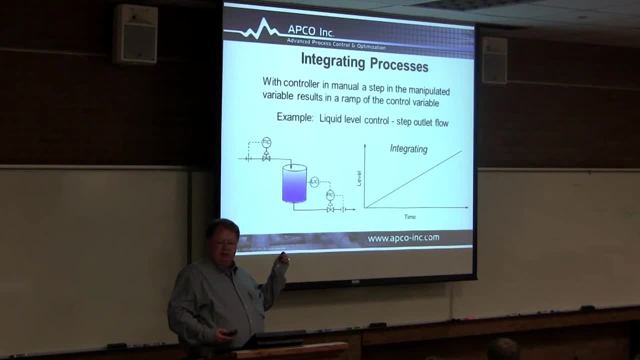 got half of the benefits on that distillation column that I told you about, Just knowing that little bit, So you can study Laplace, you can study Bode, you can study all kinds of tuning techniques that you want to, but just knowing that. 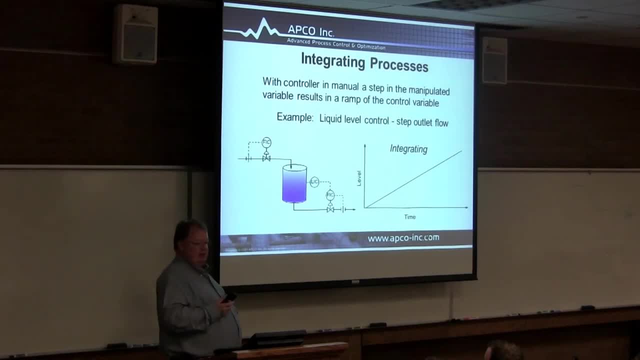 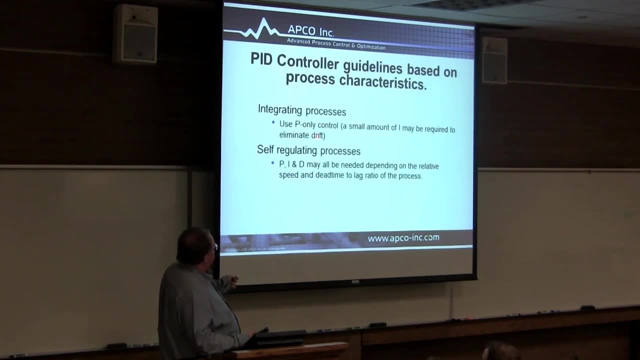 will get you most of the way there. How do you like that? Is that worth 50 minutes? Integrating process is used for proportional control. Sometimes you can use a very small amount of integral action. When I say a small amount of I, I don't mean the I value's got to be small. 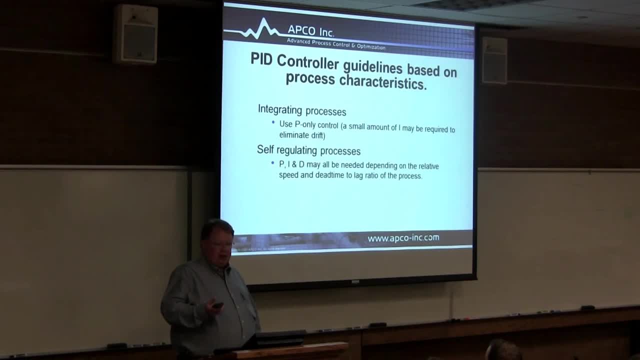 because the TI sometimes is in the denominator. If you use a small I and it's in the denominator, how much integral action do you get? A lot, So you've got to know if the I's in the numerator or the denominator. Right, I mean, we're really good engineers. 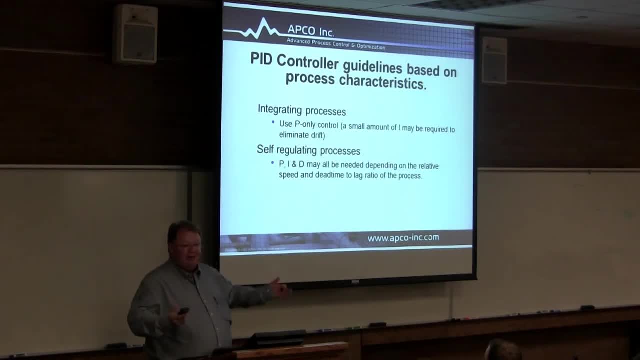 You know it's in the numerator or the denominator. It's another gotcha. If it's reset time, if they call it time, it's in the denominator. If they call it reset rate, it's in the numerator. Self-regulating property, and I give me all the units depending on the relative speed. 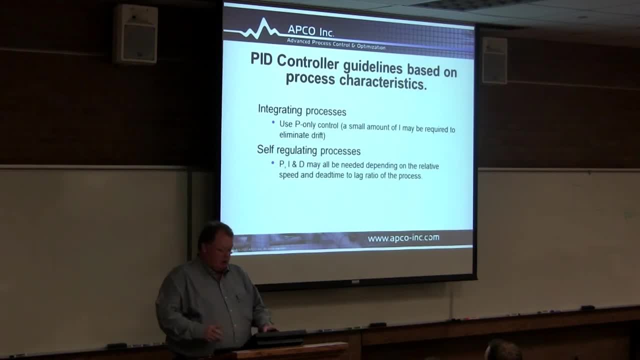 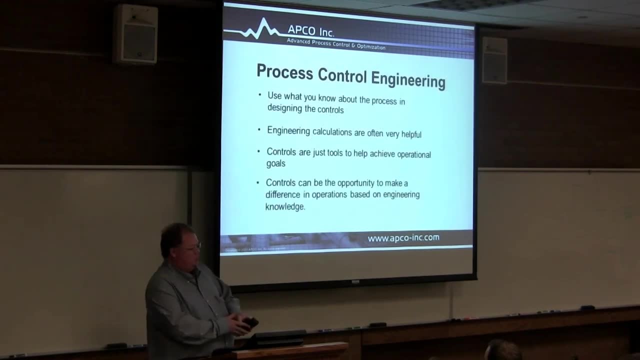 that's it. So that's it for that. Now, what I want to do is just spend the rest of the time. I can talk about that. I can talk about that, but I'm not going to. I want to spend the rest of the time answering any questions you guys have got about control. 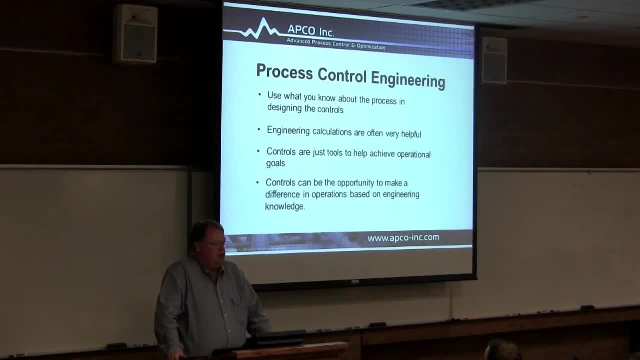 what's important, what's not important, or just engineering in general. chemical engineering We do work in just about any industry. you can think of Pharmaceutical manufacturing. so Hex-L- they make carbon fiber. we do a ton of control work out there. Three of the 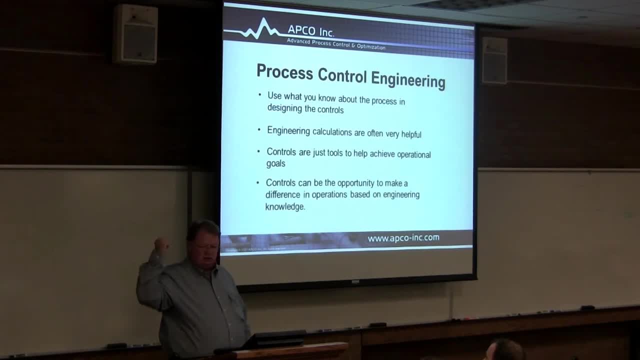 five refiners on the Wasatch Front, the water industry, the pharmaceutical industry. we make gun safes- we make you name it. we do wastewater treatment plants. we do water treatment plants, we do. we make cheese, we make dog food- we make you guys name it. 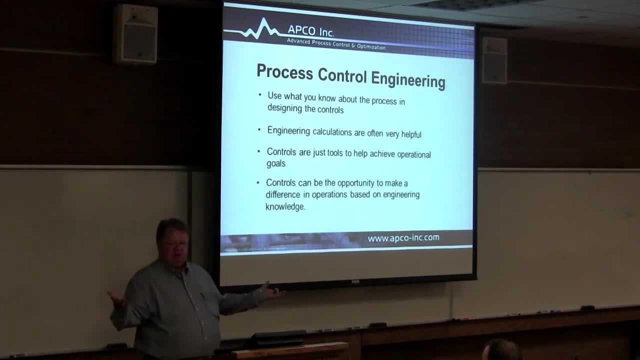 Give me anything. come on, Tell me something. you think process control or chemical engineers don't have anything to do with. Anything. come on, That's a challenge, aren't you guys? Diapers, Power bait, What Power bait. What's in power bait? 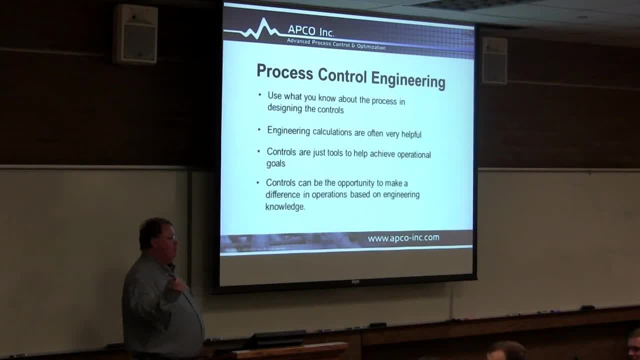 He's got a look. Chemicals- There's a lot of chemicals. There's artificial coloring, things like that. All those come from the chemical industry. right, Go ahead. What's next? Hollywood- What was that Hollywood? Hollywood? 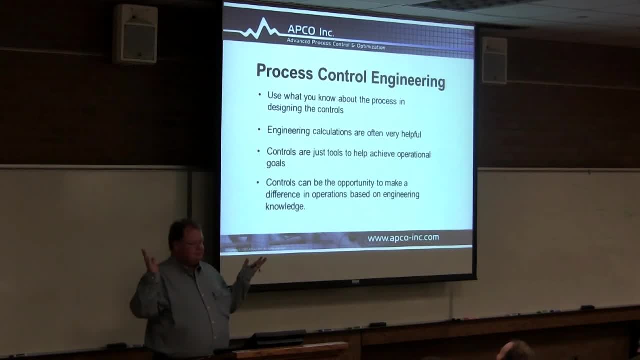 Have you seen the faces on those girls? That's all the chemical industry. What else? Anything else? You know, I did this thing at the University of Utah and somebody said prostitution, You know? and I said, come on. 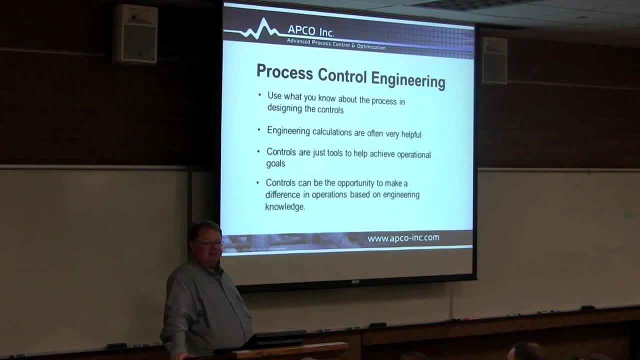 You guys, you really want me to go into all the ways that the chemicals help those prostitutes. The bearded guy in the back: Computer programmers. We use computer programmers, You know, the reality is that computer programmers are not successful at all. 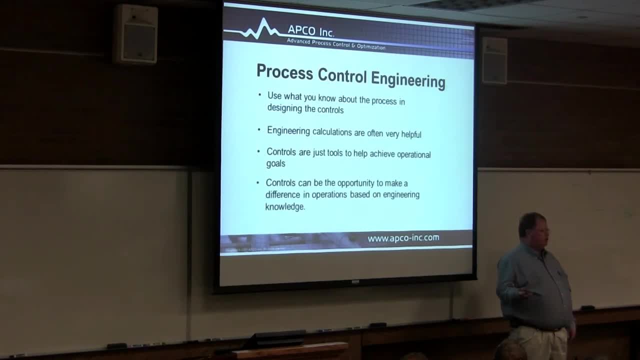 in this industry. There are some computer programmers that try to get into this industry, but they have the problem that they can do a lot of theoretical programming. They have a really, really, really difficult time knowing how to apply it to real stuff. So one of the problems that you 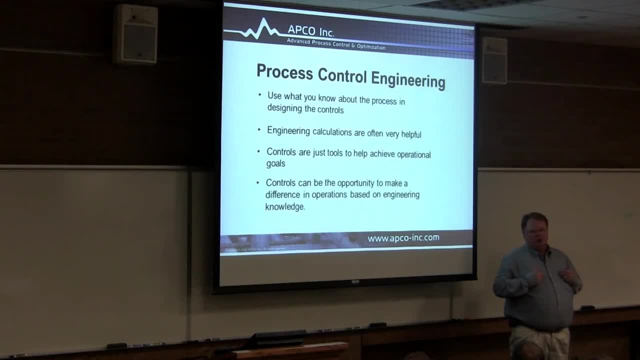 For example, in my PhD I did what I call practical process control. Practical process control is: there's a ton of theory in process control out there And there's a tremendous amount of good theory in process control, But what? What are they doing in industry? PIB control? 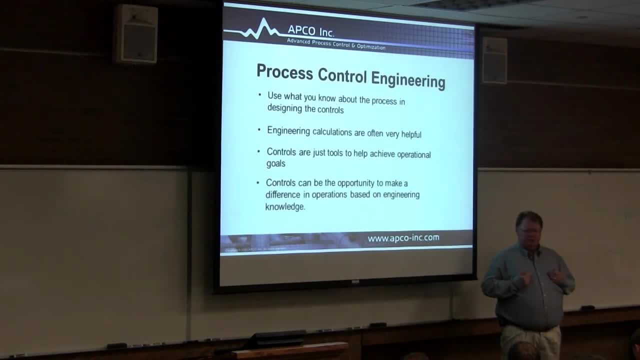 Maybe some other simple stuff. So the question is why, If there's all this great stuff, why are they using PIB on very complex processes? Why does their control stink so bad? Well, there's a huge gap. The people in industry say those people in academia they're. 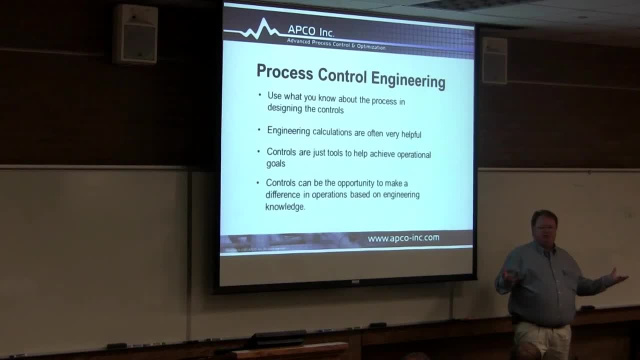 academic. If something's academic, what does that mean? Yeah, it's not real, It doesn't have any value, That's academic. So that's their perception of academia. And the academics say, wow. I remember when I got my PhD at the University of Utah there was one guy on my committee that said: 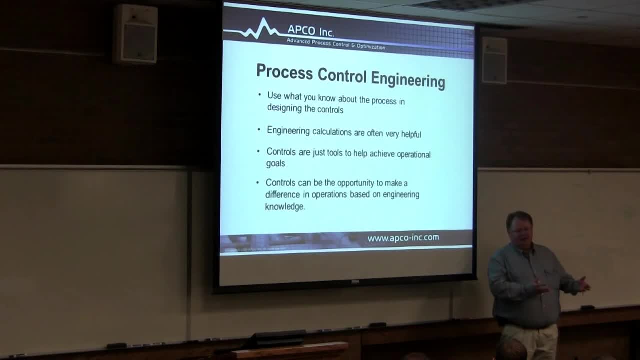 stop. So what? And that's been done in theory a hundred times, So what's the big deal of doing it in practice? That's not worth it. You see the problem with that. So there's this huge gap between theory and practice. 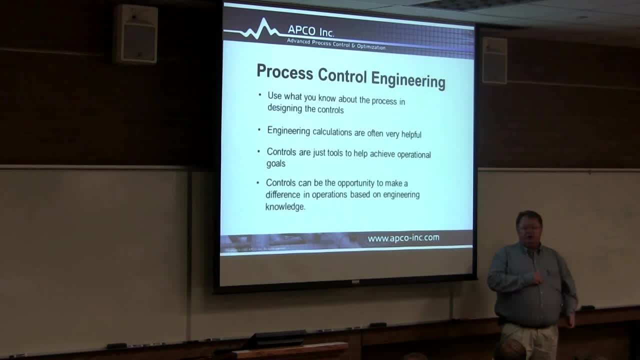 People like myself, Dr Hedegren and others are trying to close that gap. That's a huge value. Huge value Because not all processes can be controlled. with PIB control You get interactive processes, nonlinear processes, processes that are just all kinds of different things that are extremely 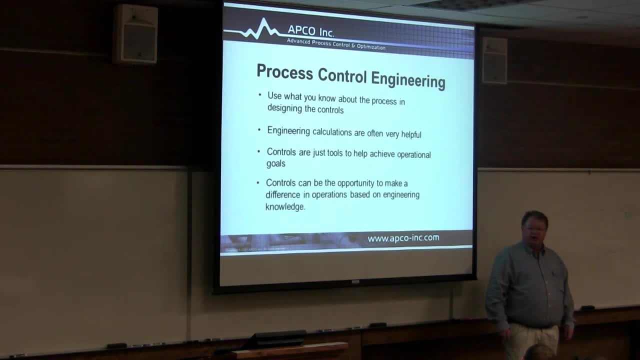 important for safety, for dollars, for quality, for all kinds of things. So does that make sense to you? So doing programming a nonlinear algorithm is something a computer science guy can do great. Knowing how to use that nonlinear algorithm and put it into an application piece of software is really something. 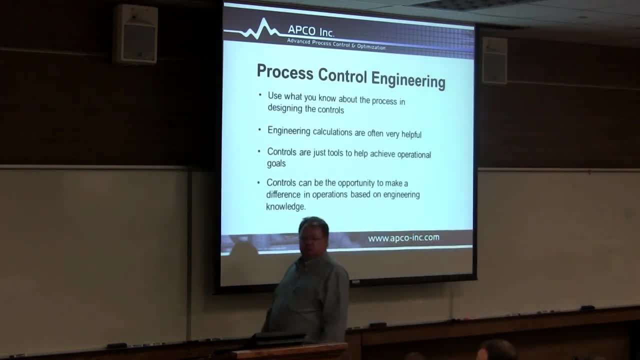 you need a good engineer to do. If someone really wants to go into process control, would you recommend that they go start off with process engineering first to get that strong background and then go to process control Or just take a job off for trying to do process control. 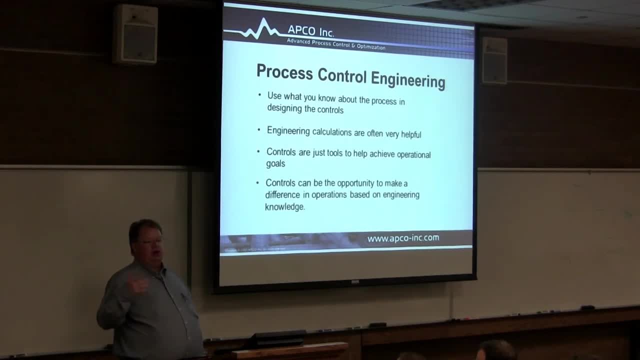 Either of the paths are okay, But if you're going to do process control, take a process control job in an industry that is doing process control on a process. At APCO we usually hire guys that have done both process and process control, So they'll start out as a process. 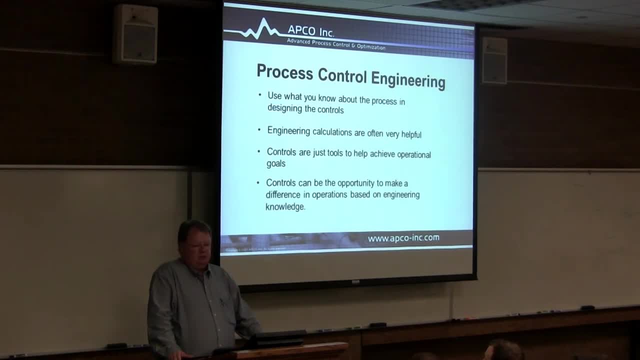 engineer or a process control engineer in a process plant, And I don't care if it's a water treatment plant, I don't care if it's a refinery, a chemical plant, a dog food plant, I don't care what plant it is, It's just so that. 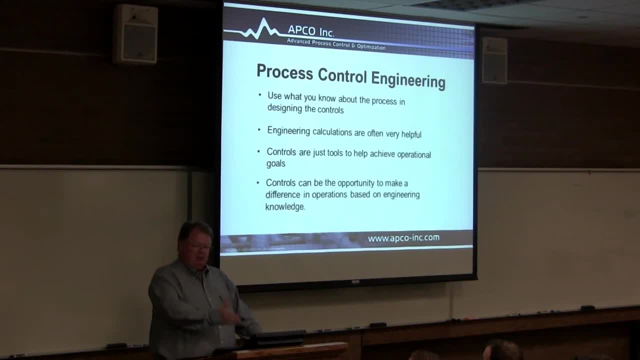 they can get used to the relationship between how to get from the computer all the way down into the process and understand how it all works together. Does that make sense to you? Do you use PLCs? Yep, we use PLCs a lot. 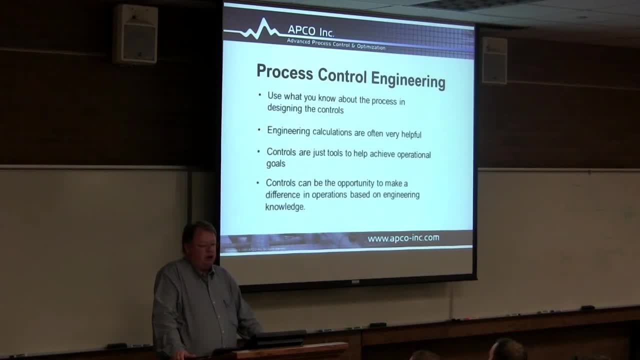 So there's two different kinds of computers used, primarily used for process control. You guys are using what are you guys using in the lab? Max LabView? LabView is not one of them. LabView is not one of them. So LabView is a PC-based control system. that's. 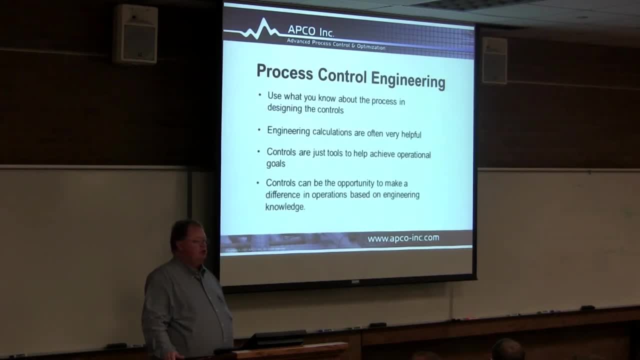 never used in industry. Never used in industry. They'll use what's called PLCs, which stands for programmable logic controllers. There's a hundred different kinds out there. One of them is called Rockwell. One of the things I'm thinking about doing is Rockwell has approached me about making a gift. 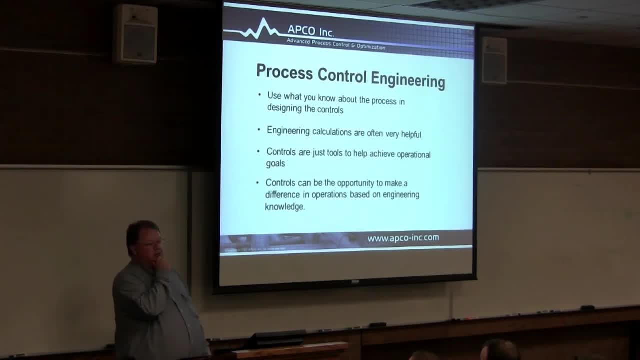 to the chemical engineering department here to put them in their lab, And I have to talk to someone about that to see if they want to do it. The problem is you have to have somebody to implement it. But that's a real industrial system. That's what's going. 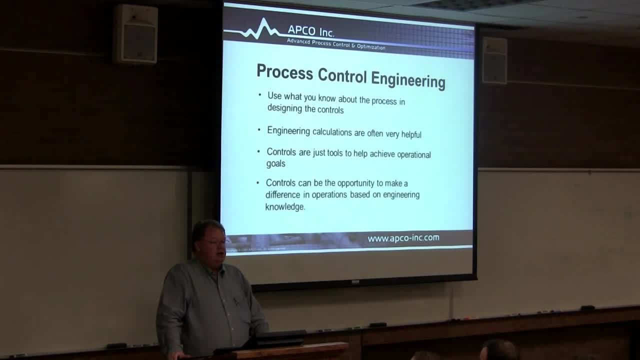 into the Big Western refinery. right now It's being swapped out. The other kind of system is called a DCS distributed control system. That's historically a much bigger system like the Bailey system was Now the Bailey system's 25 years old. So you wouldn't expect a computer 25 years old to be great, right? 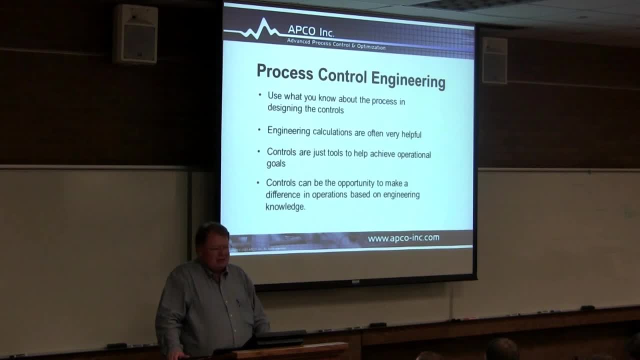 So anyone who worked on the Bailey's- oh, it stinks so bad. I said, yeah, well, fire up your computer from 25 years ago. Tell me how good it is. These control systems are very much tied to the computer industry. 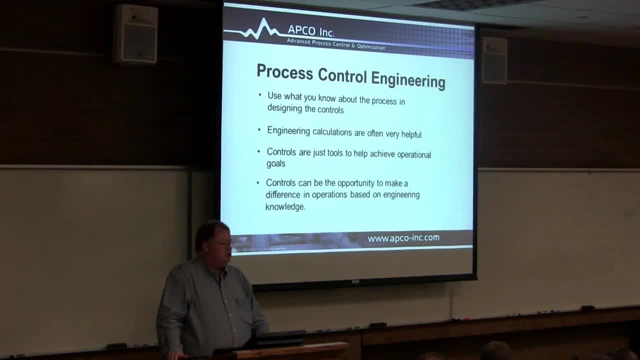 And so after a decade or so, 10 to 15 years, you need to replace these, And that's just the way they work: PLCs, and so you learn programming languages. associated with PLCs, There's IEEE 11,, 5,, 16,, 1, dash. 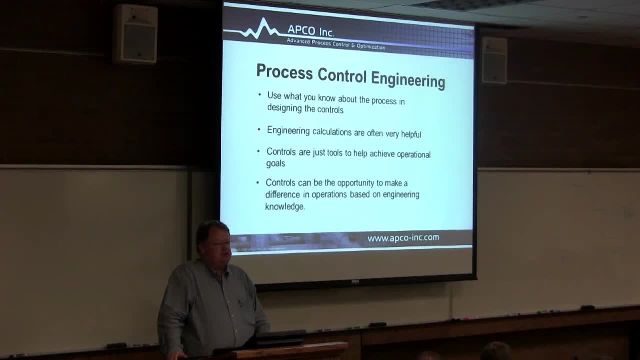 blah, blah, blah, blah blah. There's a language that has six languages that you can program in there And you do a tremendous amount of work in those Boil gas industry. that's also areas we work in, Anything else. 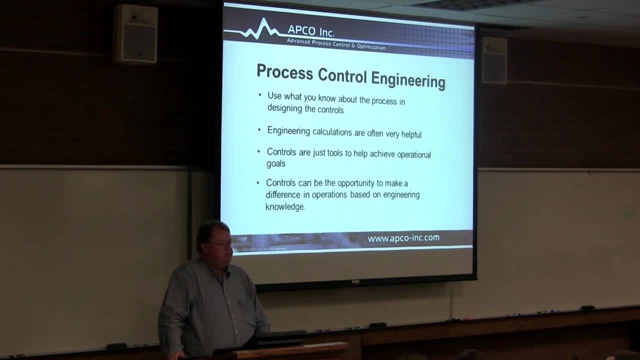 Any other questions? Don't you guys want to ask how much you make A process control engineer? If you're a good process control engineer, I could get you a job anywhere on the WASAT front for making pot dollars. So I've got a friend of mine that's been out of school for about 10 years. 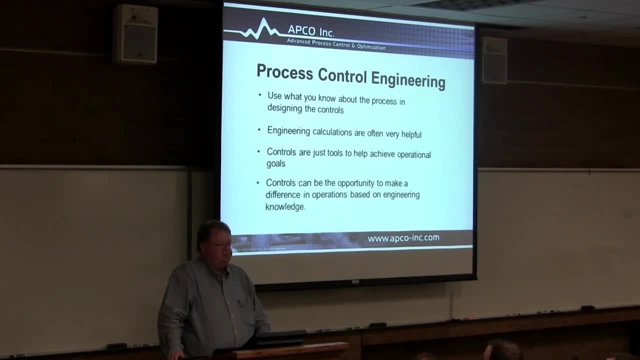 He's making about $125,000 a year. The reason: there's always positions open in process control, Always, always, always, always, And it's because it's a little more difficult than your steady state calculations. you're doing the heat transfer. 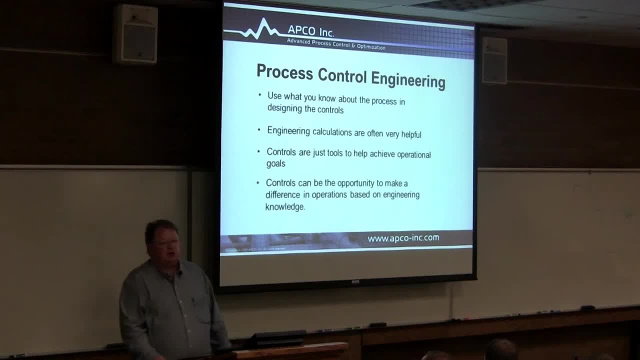 mass transfer, things like that. You have to deal with that. Any other questions? Thank you, guys, very much, Thank you.